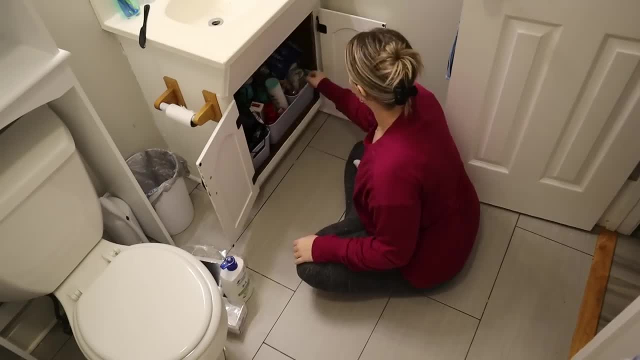 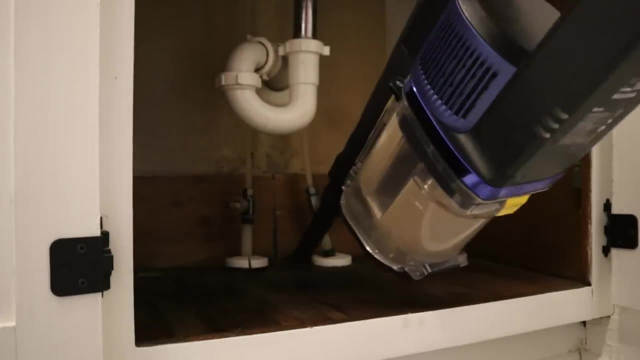 everything into categories so I can figure out where I want to put everything. and it does take a little bit of trial and error to figure out how everything is going to fit and how everything is going to work out the best. So you might see me moving things around a little bit and underneath. 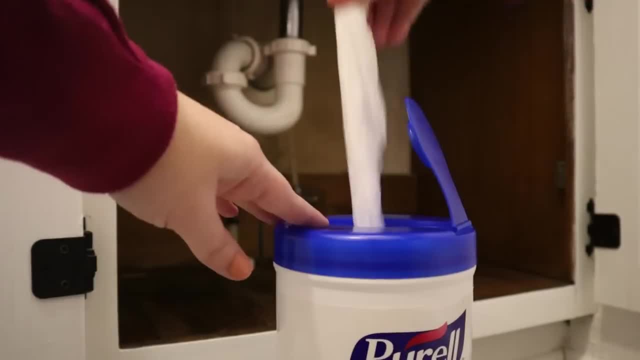 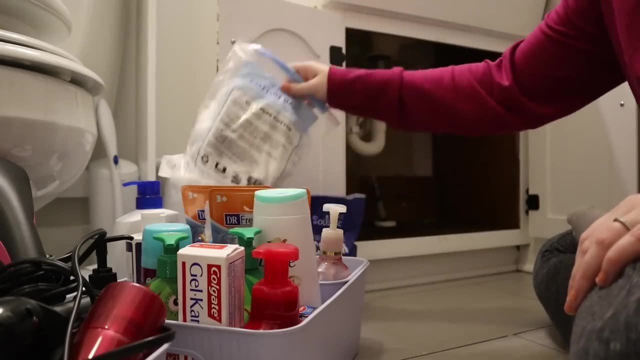 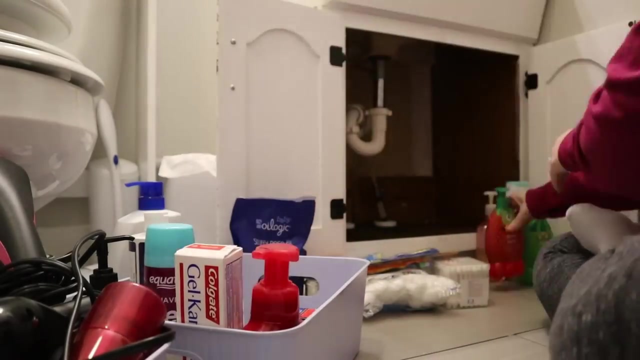 this cabinet is in kind of bad condition, So I just do my best to take care of it in the best way that I can. So we're going to go ahead and wipe it down and figure out how I can store all of this. Also, all of the organization that you see me using in this video is organization that. 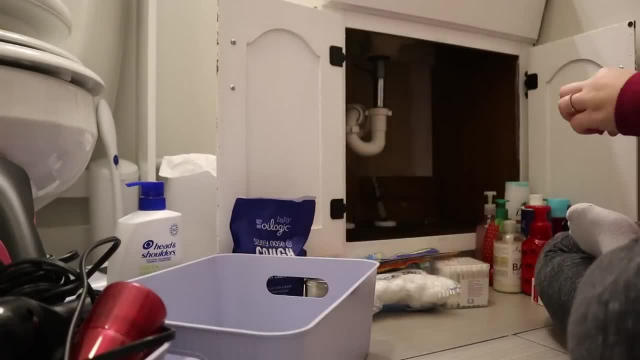 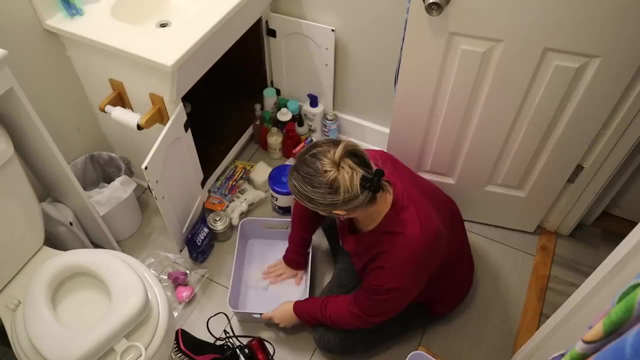 I've already had or things that I have recently picked up from Goodwill, So I'm so excited to show you all the way that it turned out. It turned out so good. The bathroom actually ends up looking bigger without that gray shelf in here, and I found a. 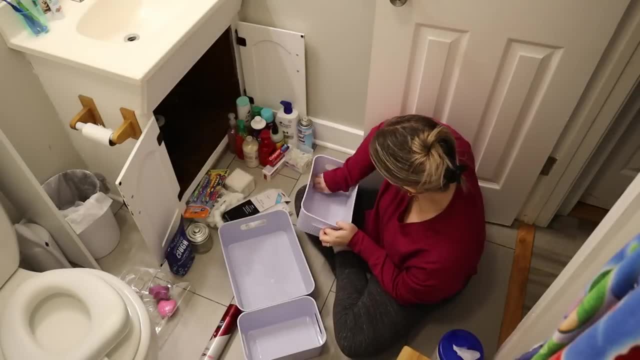 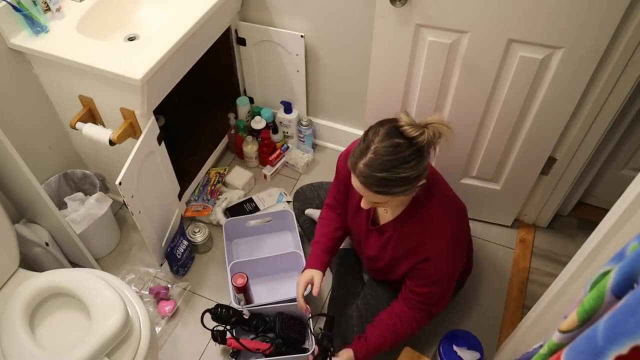 beautiful mirror that I'm going to be hanging in here over the top of where the kids hang their towels. But I already had these little organizers down here. I got these from Five Below. They were five and three dollars. The large one was five dollars and the two smaller ones was three dollars. 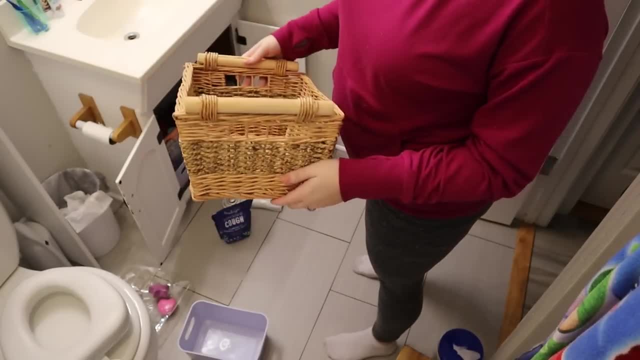 So it did take me a minute to just kind of figure out how everything was going to fit, and under the sink I just have a few extras that I end up taking out and storing in this basket here. I got this basket from Goodwill and I'm going to go ahead and put everything in here. 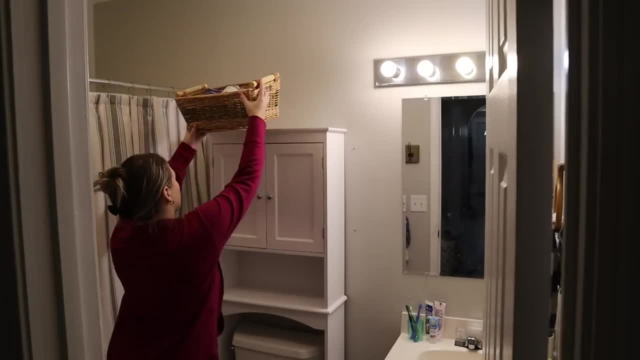 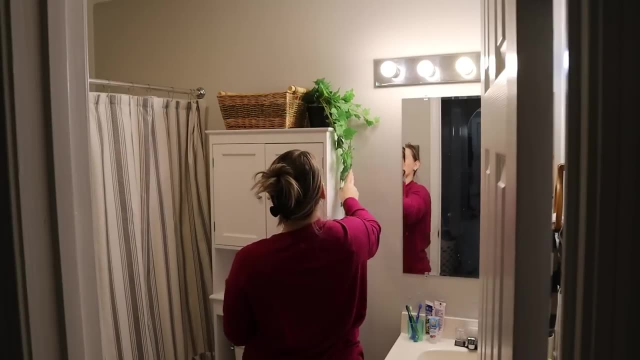 I got this basket at Goodwill recently for $4.99.. It was a steal of a deal. I love finding my baskets at Goodwill, But anyways, all of the extras that I was keeping under the sink, extras as in shampoos. 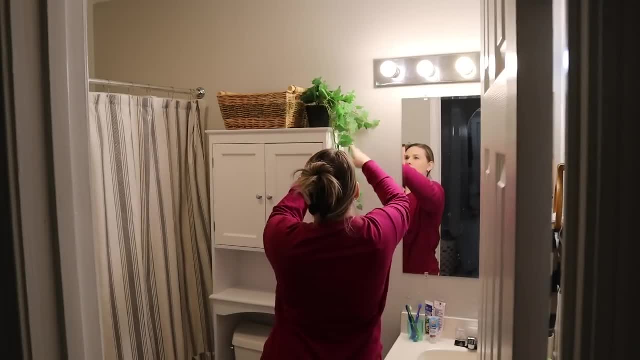 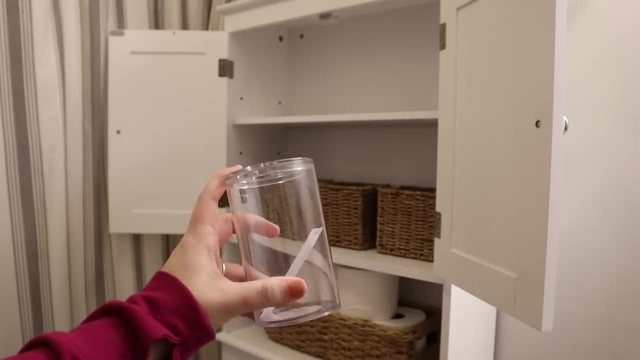 and toothpaste that are just extra for when we run out. I want to store in this basket and put it up high, because it's not really something we reach for every day. So things that the kids reach for every day I want to put down low, And I did find these acrylic toothbrush holders from Walmart. 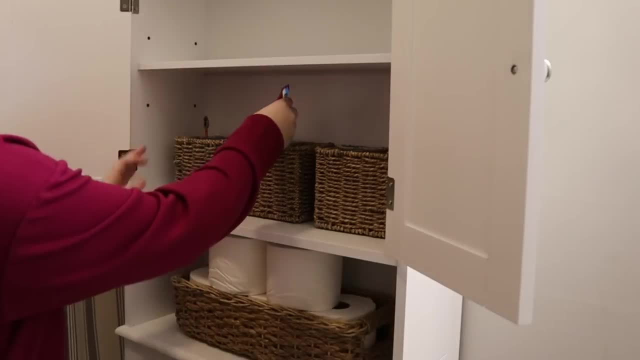 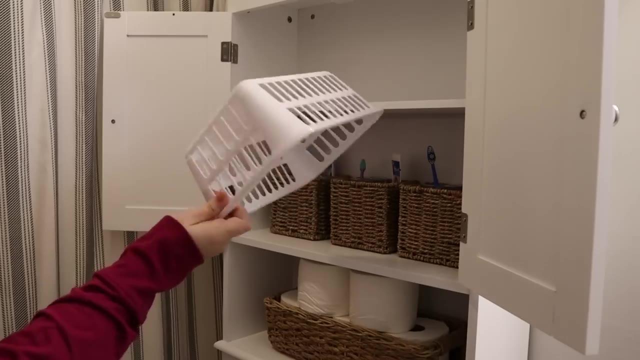 for two dollars a piece and I'm going to go ahead and put them in these Goodwill baskets and it just makes them look prettier because they're in baskets. I love to use baskets around my house. It just makes my home feel warm and cozy. I'm also going to be adding this white basket up here that. 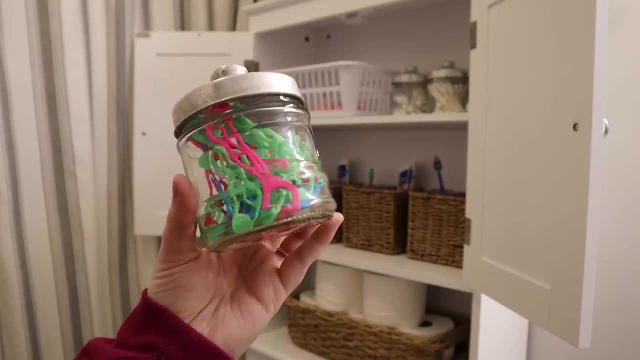 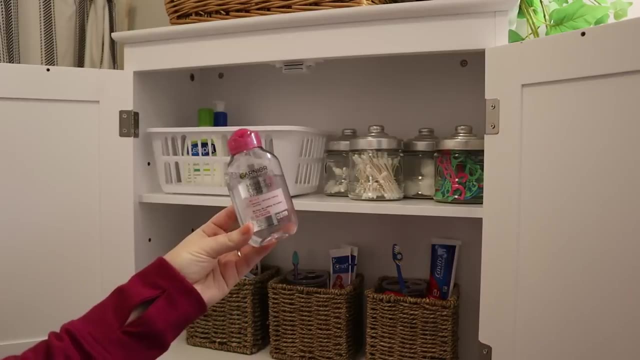 was two dollars from Walmart and three of these glass jars that I've had for years. I found these at the Dollar General forever ago and I just have q-tips and cotton balls and toothpicks And over here in this white basket. I'm actually going to switch this white basket out for a gray basket. 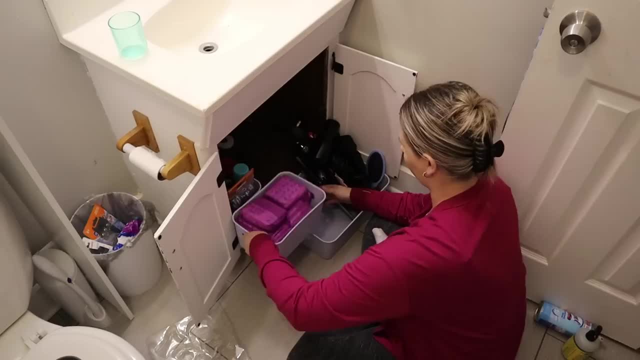 because when I closed the doors the white basket did not fit very well. I kind of had to push the door closed pretty hard. So I'm going to put these in here and I'm going to put them in here Hard for it to close all the way. So I'm going to actually switch that out here in just a little. 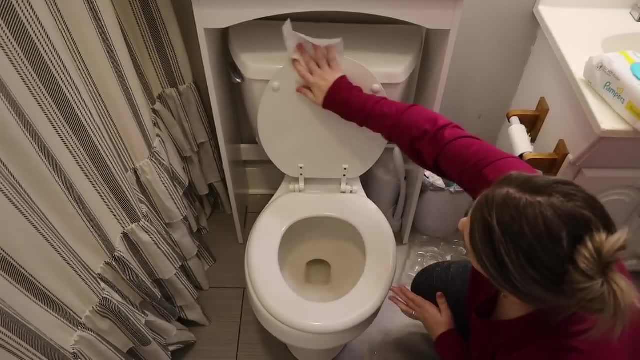 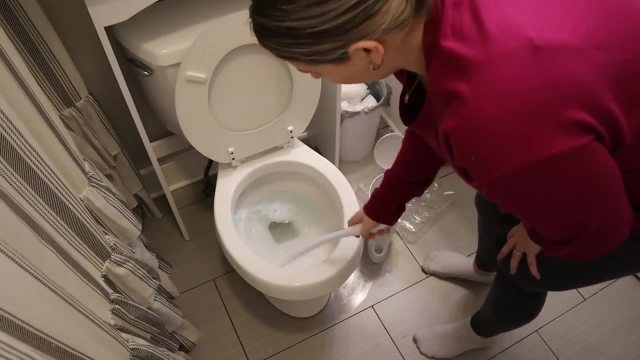 bit, But I'm using that basket for my 13 year old's things because she is older, so she needs to have her own personal basket in there for her face wash and her moisturizers and her acne treatment and things like that. So I did have a designated space for her to keep all those things. I didn't. 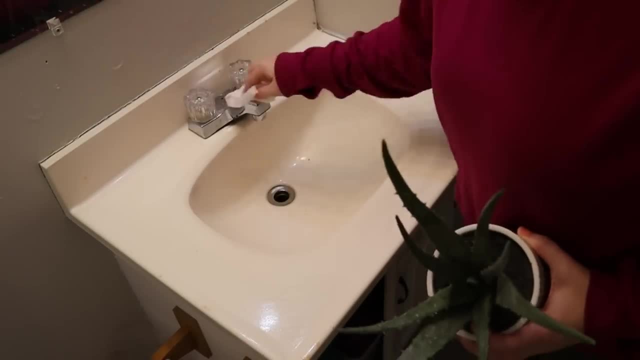 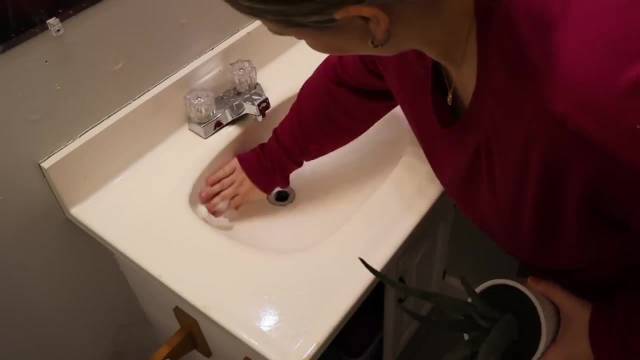 want to go out and buy a whole bunch of new organizers for my house, So I did use things that I already had around my house or things that I found cheap at Goodwill. The only thing I really bought new was the bathroom cabinet, because we really needed a storage cabinet in. 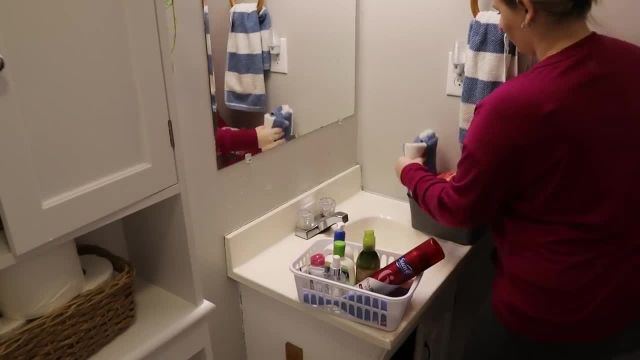 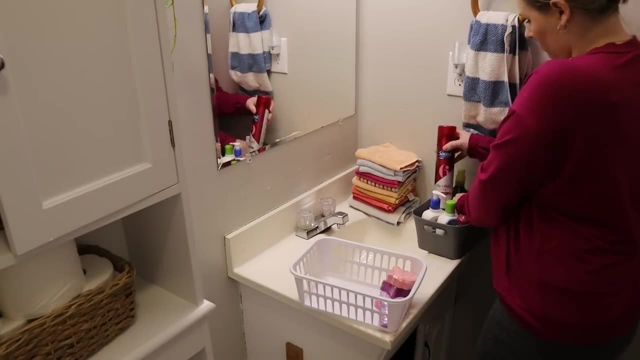 this bathroom. I struggle so bad with storage in this bathroom with four kids. So here I'm just going to use this gray basket to put all of my 13 year old's things in, And I'm going to use something else for the rags, And I'll show you guys the way that I organized everything here at. 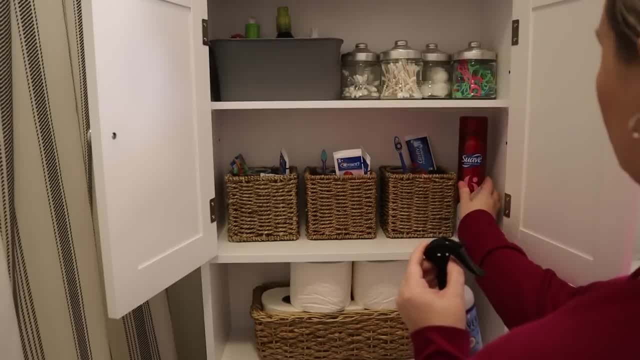 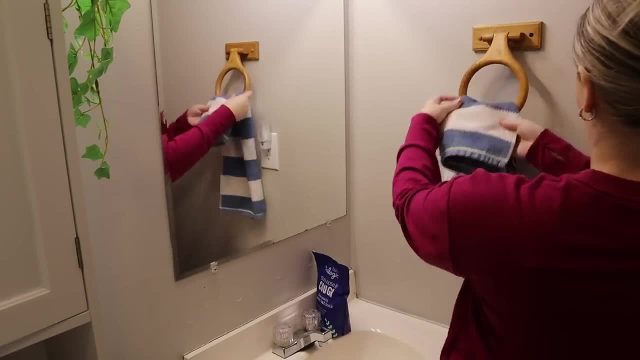 the end, But it ended up working out so much better than that gray organizer I had in here. If you guys are subscribers, I'm sure you have seen it or you've seen me take it out of the room before I started putting things in this white organizer. We're also going to add some. 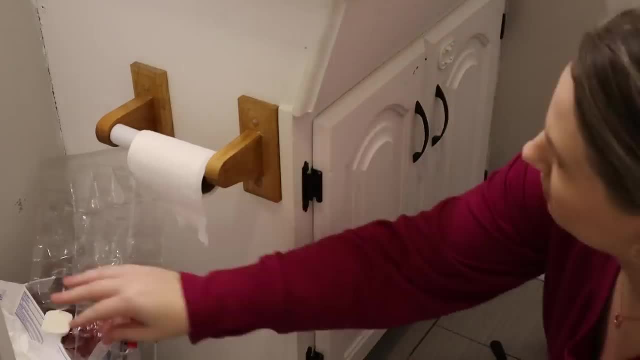 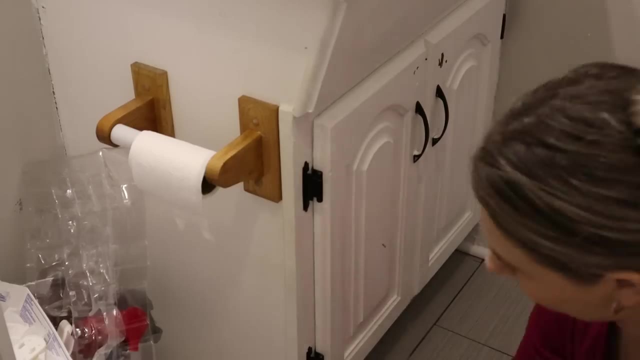 strawberry pound cake bath and body works, hand soap over here on the sink. That stuff smells so, so good. I'm going to pry off this baby lock that was on the cabinet because it was broken and it did rip off some of the paint. I recently had painted this cabinet white because it was in. 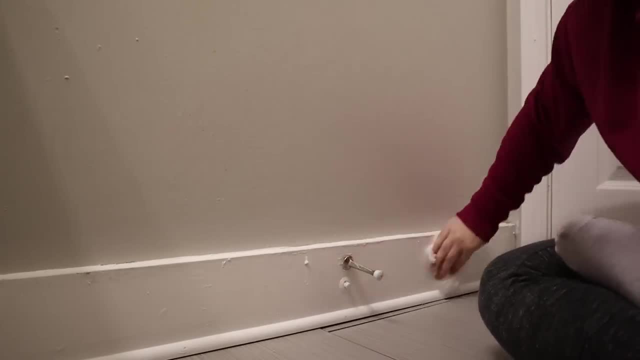 terrible condition. But I can just touch up that later and fix the paint. And I'm also going to wipe down the bottom of the walls and the baseboards because my kids just like to touch the walls with dirty paint. So I'm going to wipe down the bottom of the walls and the baseboards. 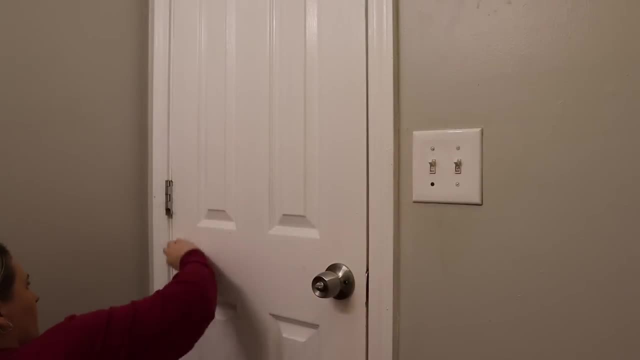 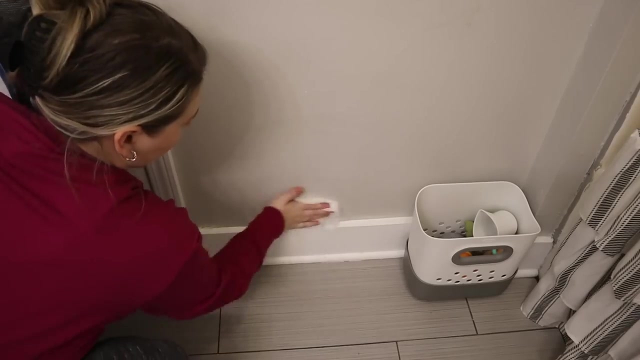 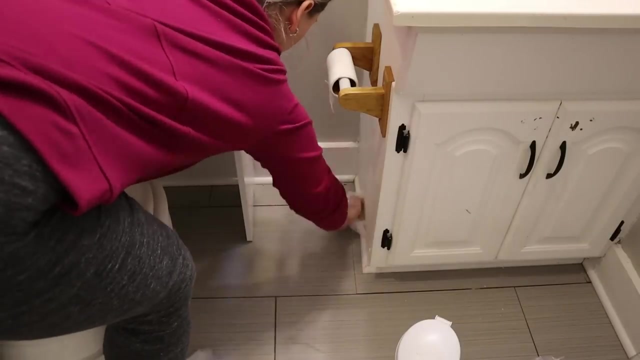 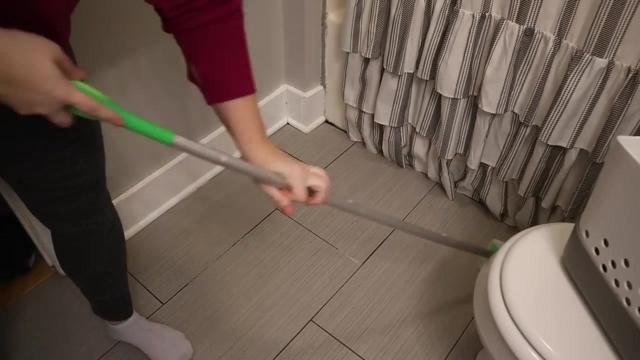 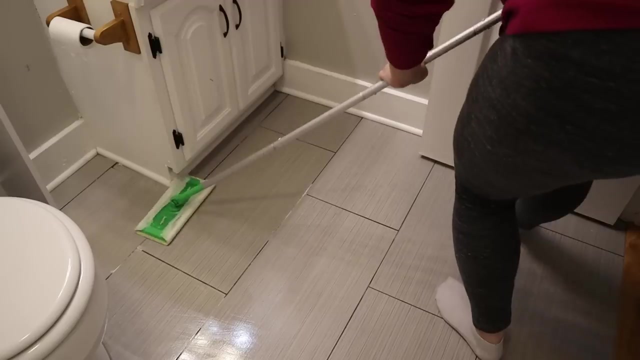 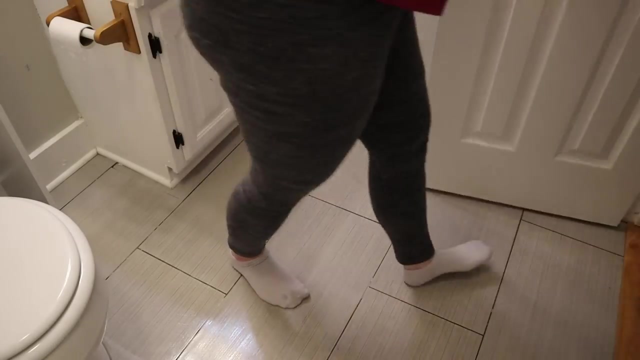 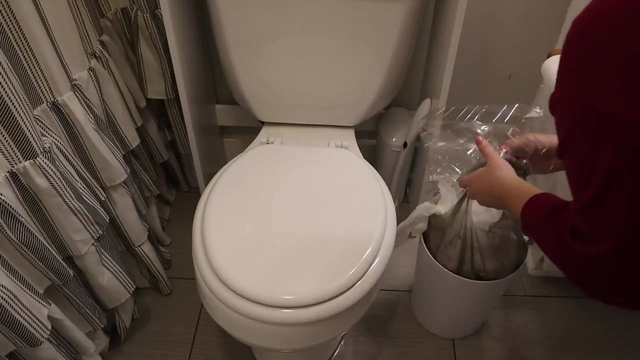 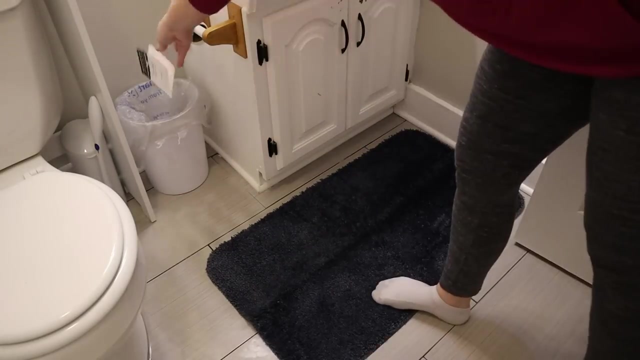 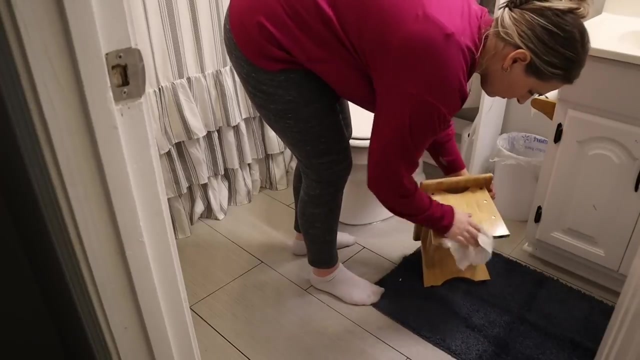 and put their feet on the walls. So we're going to get this all taken care of. I picked up this rug for the kids bathroom. It was about $13.. They had a little yellow flower rug in here, but it slides around too easily, So I'm going to put it in the bathroom And I'm going to 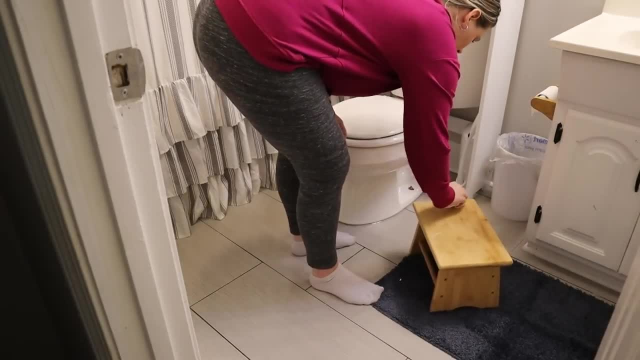 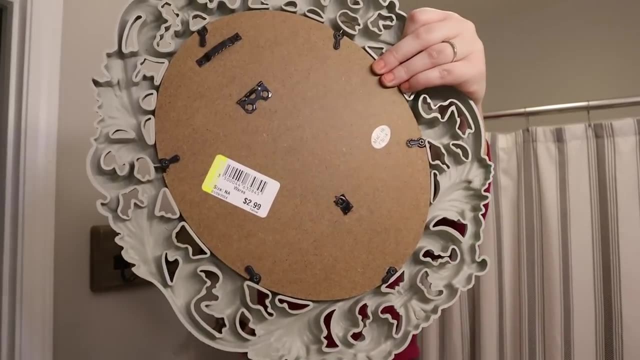 and it was always scrunched up and I just got tired of it. So I broke down and bought this dark blue rug because it matches the shower curtain. As you can see, it kind of has dark blue navy stripes, And I found this mirror for $2.99 at Goodwill and I thought it was absolutely. 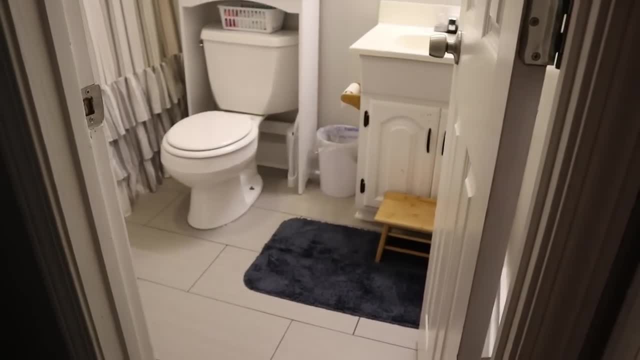 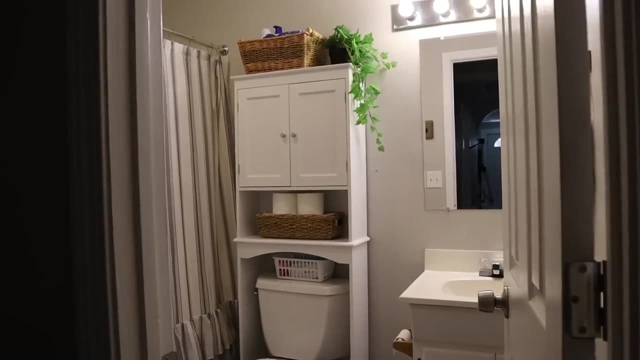 gorgeous, So I wanted to use it in the kids bathroom and I have the hooks on the wall for the kids to hang their towels up. So I just went ahead and hung that mirror over those hooks And this is the way the bathroom looks after I love it so much: The tall cabinet and the mirror. 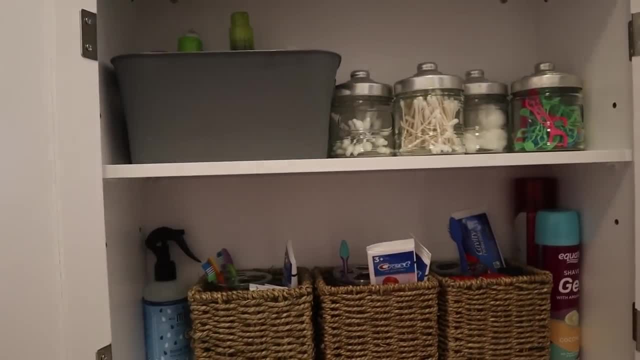 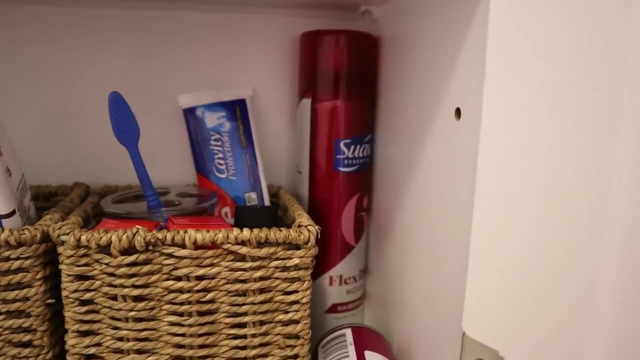 hooks makes the bathroom just look taller and bigger. Everything is so organized And you know sometimes it's more about everything looking so aesthetic. You can make things look nice, but they don't have to be 100% aesthetic. So I have my daughter's shave cream and hairspray in here next. 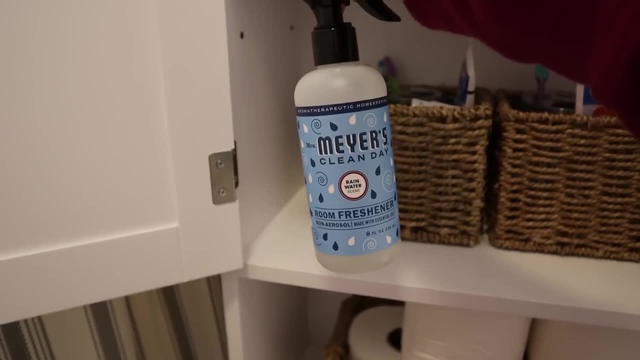 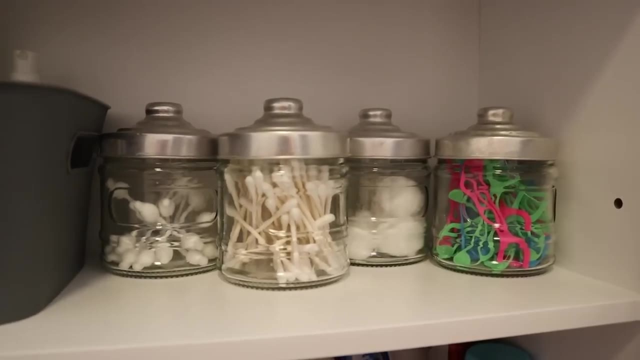 to her toothbrush basket. The middle basket is my six-year-old's basket And the last basket over to the left is my boys basket. They share one for their toothbrushes and toothpastes. Then I have the rainwater scented air freshener next to that. That smells. 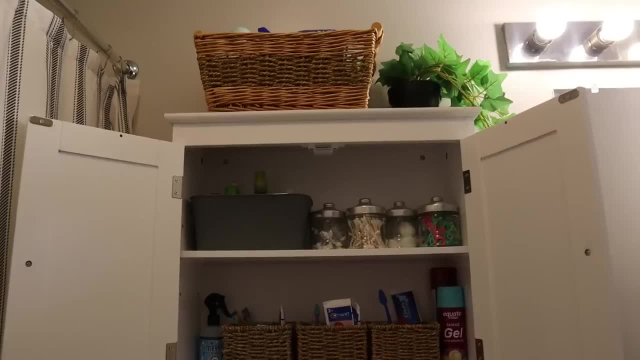 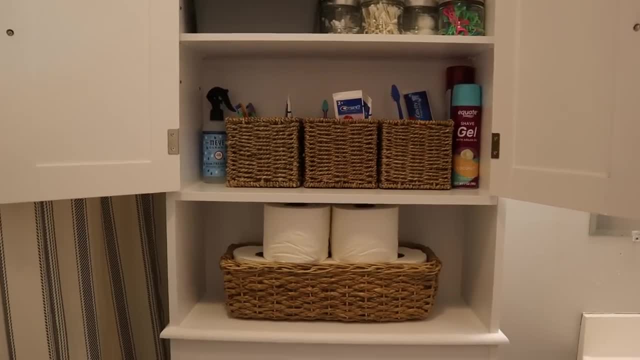 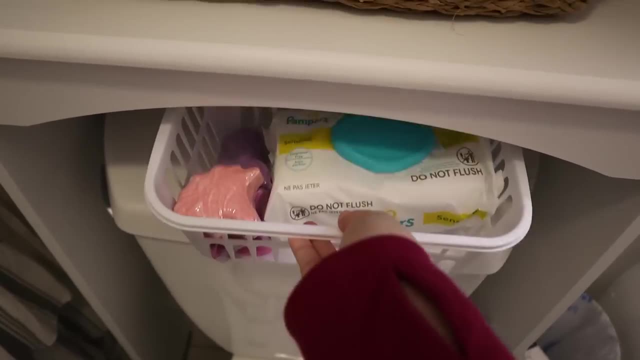 their floss and everything they're going to need hid away in this cabinet. It also looks very neat and tidy, And then I also keep the toilet paper here for extra toilet paper. And then in this basket I just added some bath bombs and some baby wipes for the kiddos, And I just love how neat and 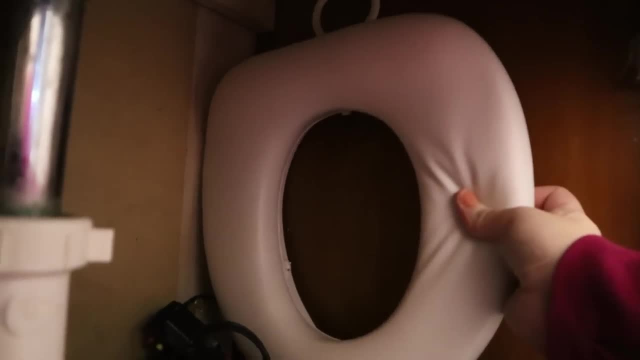 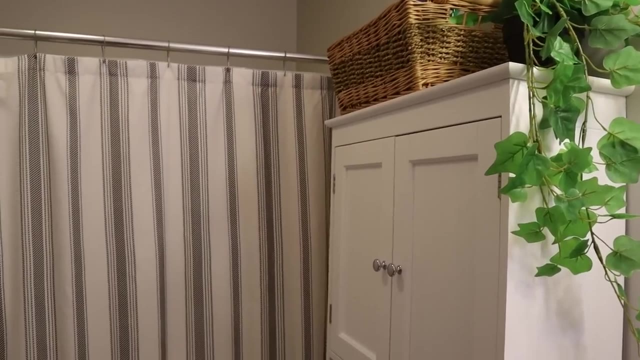 organized it looked. And then underneath the kids bathroom sink, I'm gonna get a command hook to hang this potty seat up here. I've used this for all my kids and I just kind of am saving it for when I body train my two-year-old. We have not got there yet, But I'm gonna get a command hook so I can hang. 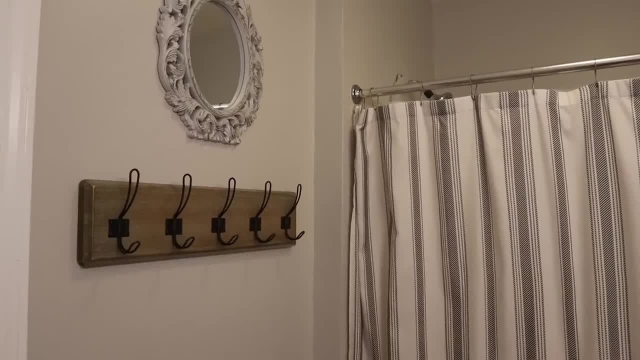 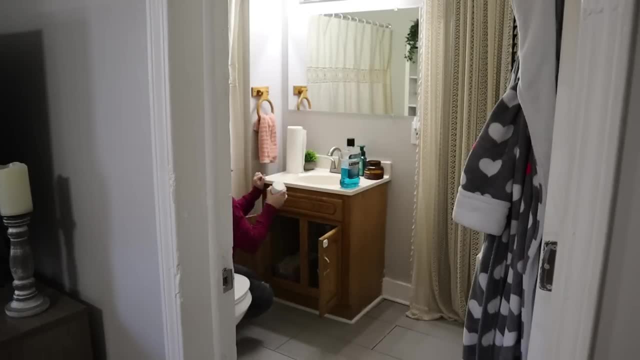 that up underneath the cabinet right there to get it off of everything that's under there. But I love, love, love the way that it all turned out. And next we are gonna head into my bathroom and go ahead and pull everything out from underneath my sink, vacuum it out, wipe it down and reorganize it way. 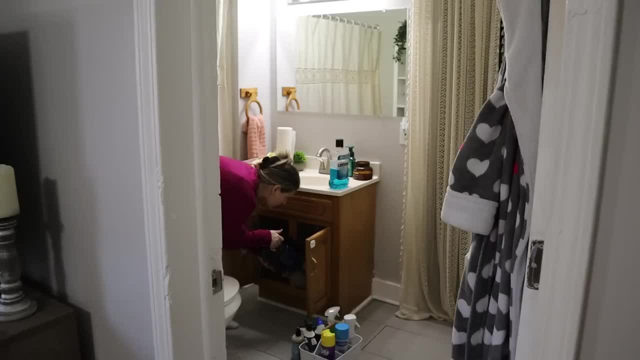 better than it was in there. You'll have to let me know: do you have like a cleaning closet or do you keep all of your cleaning supplies in a designated area like underneath your kitchen sink or in your laundry room? I really have not figured out where I want to keep all of my cleaning supplies yet. I really need to. 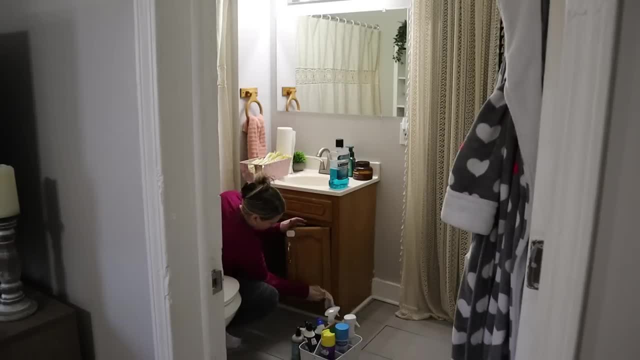 figure that out. I don't really have room for a cleaning closet or just a cleaning area to keep everything, So I just have this little caddy here that I will store underneath my bathroom sink, And I wanted to take that out and put it somewhere else because I don't like it to be under there. 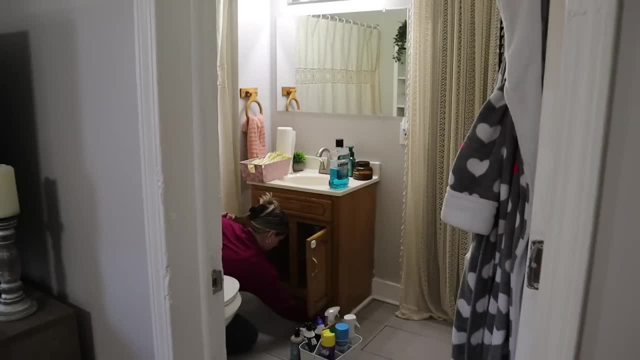 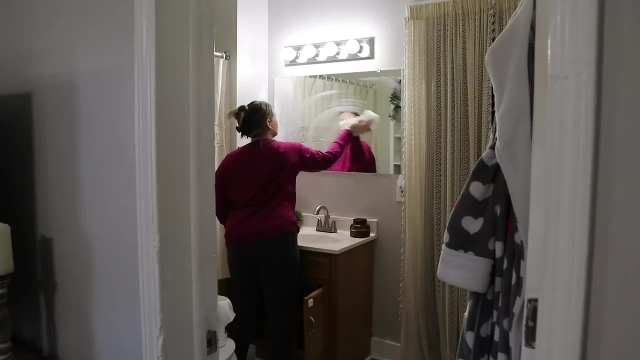 with my everyday things like our mouthwash and just stuff that we keep in the bathroom. I don't really want to keep our cleaning supplies down there with it, So I'm gonna take that out and just go start my kitchen until I can figure out what to do with that. 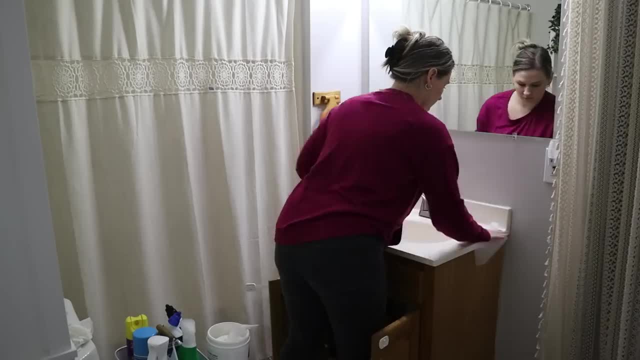 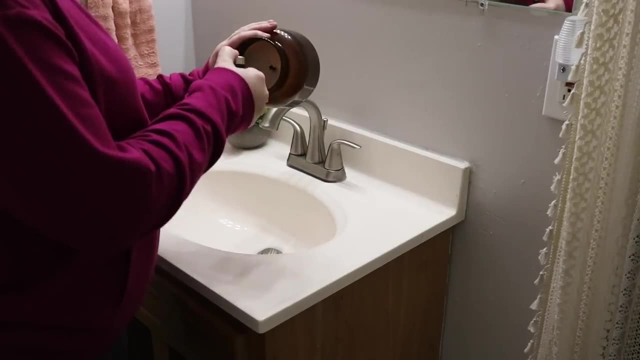 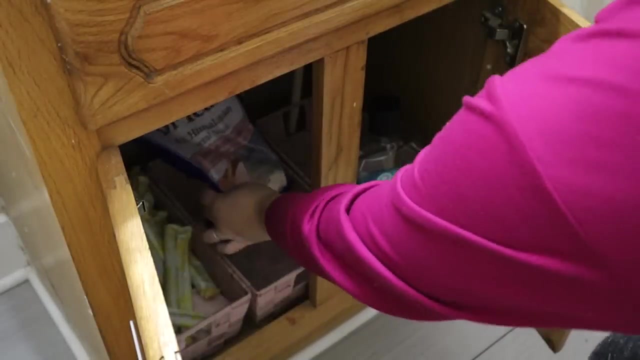 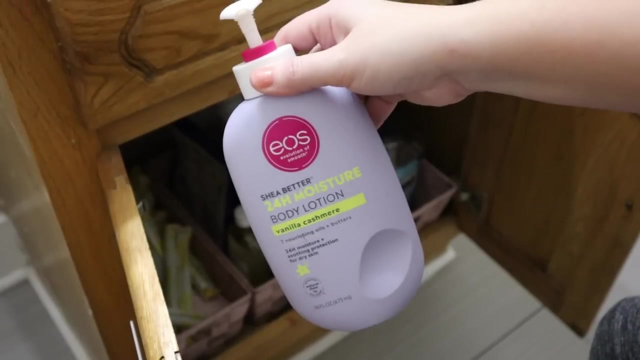 But hopefully I can come up with a good idea for a one day cleaning closet or a cleaning space to keep all my cleaners there. I'm using three baskets that I already had for underneath my sink And I'm just putting in my personal items like my tampons, panty liner, some bubble bath, some lotion. any tanning, anything else, that I don't have all the cleaning supplies have. I'm also going to be putting in a few sand Palestinian盆 in here for my customers, And I'm also going to put some sprays of dissecting, because they gave me a loaf of additional Boys and Sleep stuffs, So I think it's going to be a lot more fun, But I'm really excited about these items. 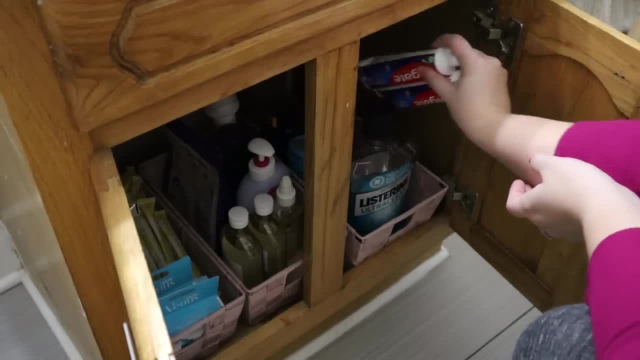 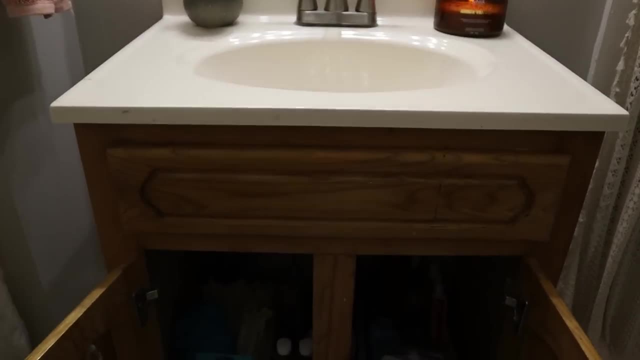 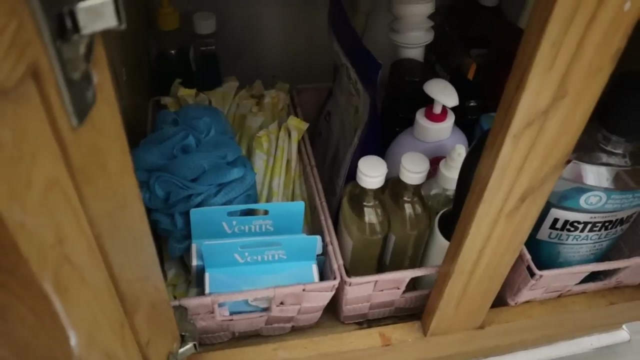 tanning aloe razors, mouthwash, extra toothpaste, extra body washes, anything like that. I'm going to be storing it underneath my sink and behind the pink baskets there's a little gap, a little space, so that I can add more things. So back there I just put my aloe and I also put my peroxide and 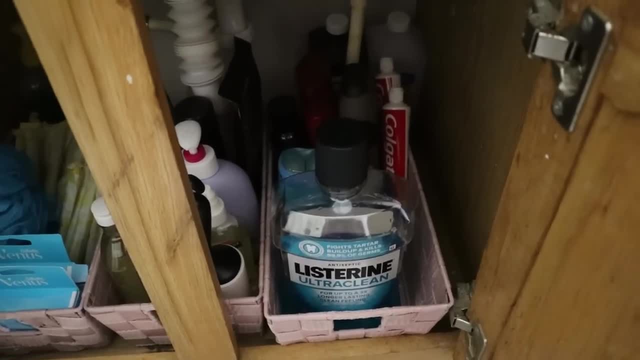 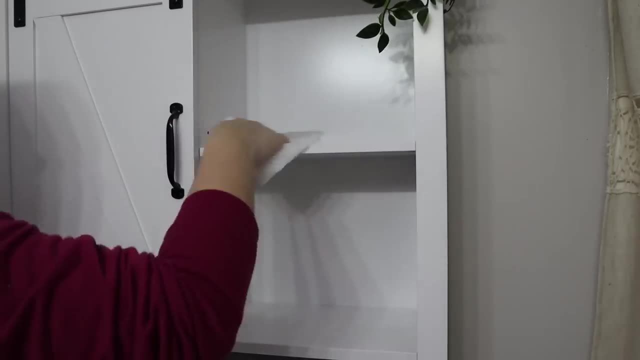 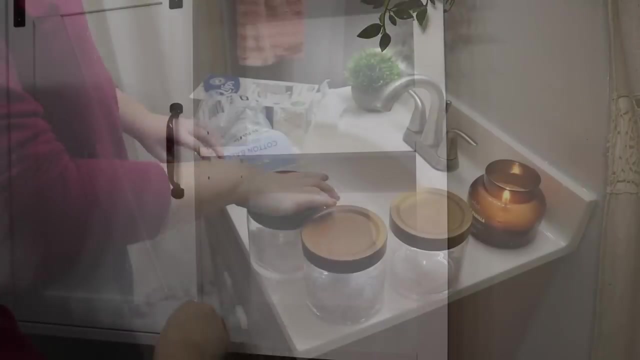 my alcohol back there so I can store a few more things in the very back that I don't reach for every single day. And my over the toilet cabinet is different from the kids. The kids have two doors that close all the way. I wanted theirs to be like that because I've got four kids sharing. 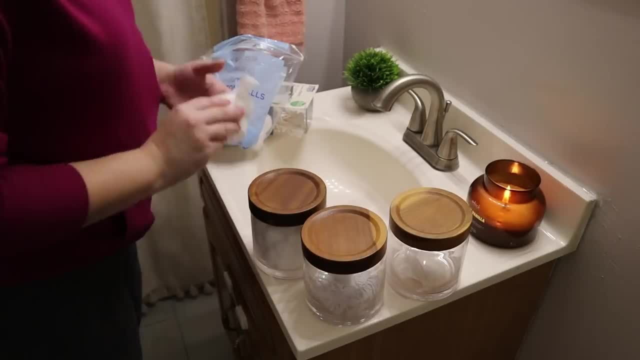 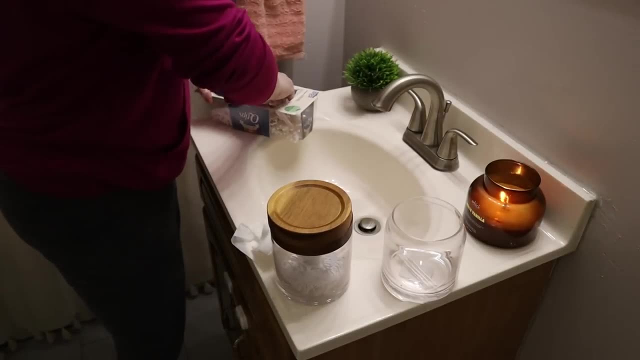 that bathroom, so I knew I was going to need all of the space For the cabinet over my bathroom. it's a sliding door so there's only one side that I keep all of our stuff in, and then the other side. I want to make it just look nicer without storing a whole bunch of stuff like colorful 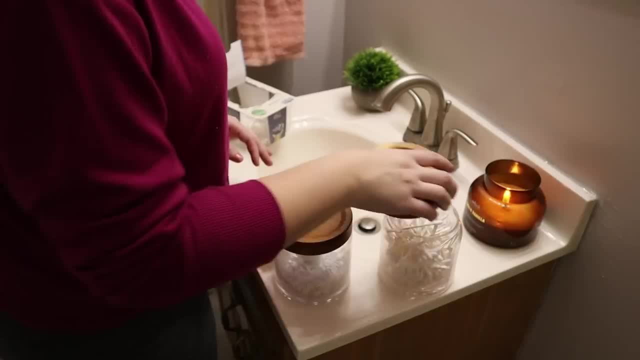 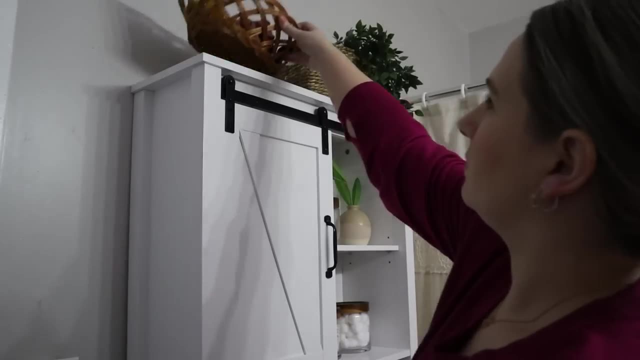 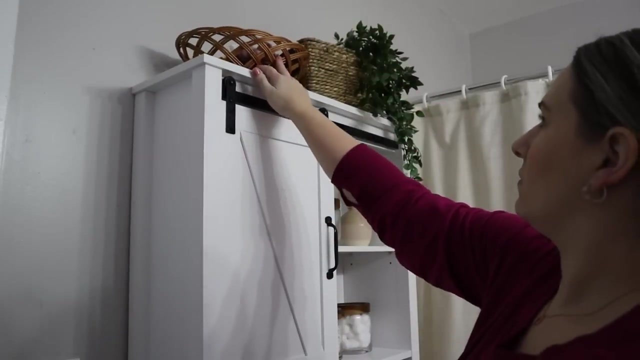 bottles of lotions and stuff on the shelves. So I like to use these really pretty glasses that I got from Target a while back to keep my q-tips and cotton balls and things in and floss, and I just added a foot file underneath my sink that I had found And then on top of my cabinet I keep this. 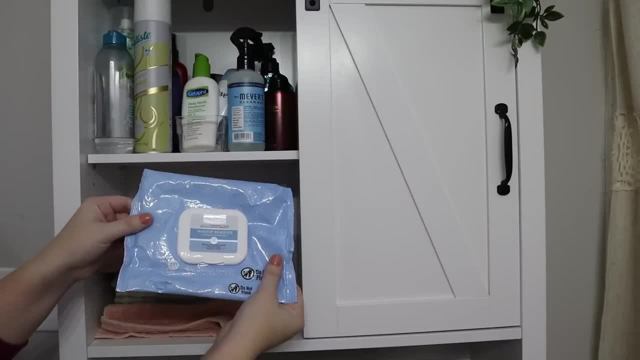 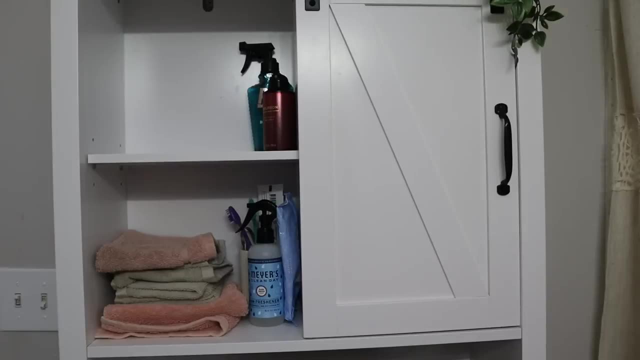 basket with all my hair bows and my claw clips and then in here I'm just showing y'all this is where I keep my makeup remover wipes- which those are almost gone. I keep our air freshener, our bathroom rags, our toothbrushes, and then up on the top shelf. 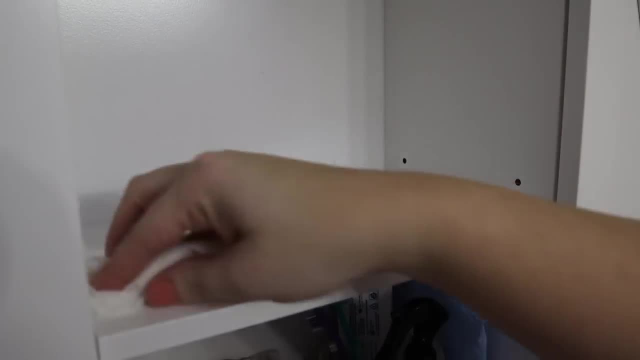 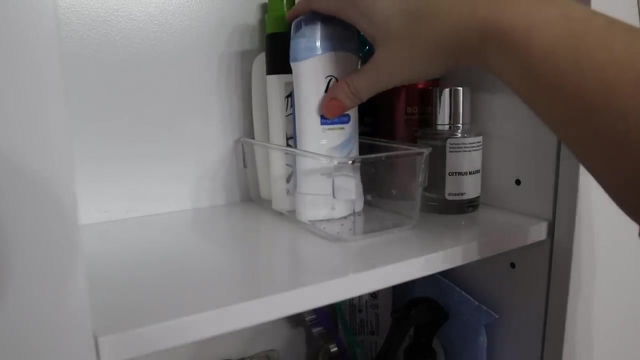 the right side is my husband's everyday things like his cologne and things that he just uses every day, which is pretty much just his cologne. So he's got three colognes and then I have a little container with my deodorant, my face moisturizer, my hair oil, my dry shampoos. 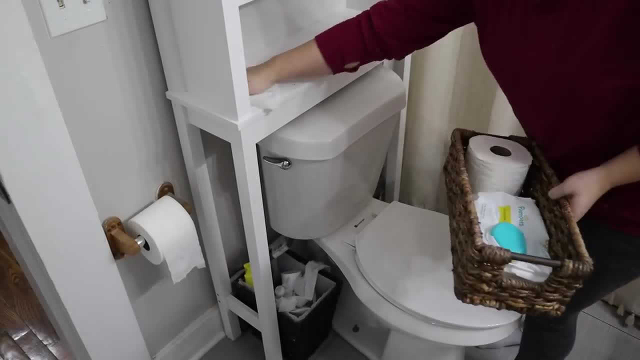 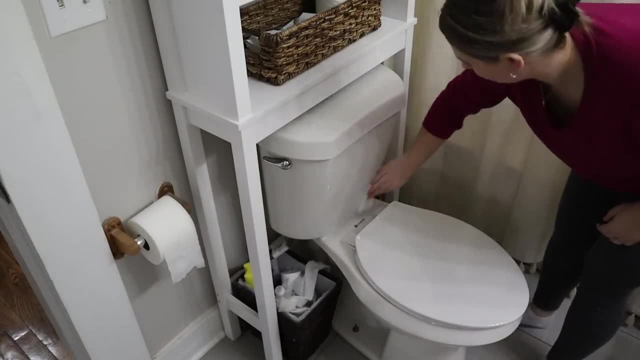 all of my hair stuff. So we're just gonna keep that up there and obviously my side is bigger because I have more stuff. He's just simple and has just cologne, but also we have a big organizer in our closet. He has a lot of our stuff, which, by the way, I'm gonna be doing a spring cleaning series coming. 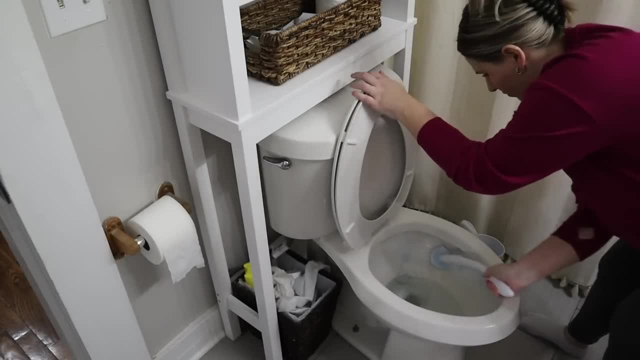 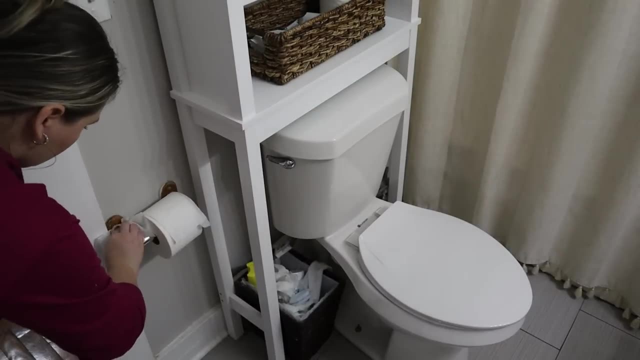 really soon in February, I'm gonna be tackling spaces in my home. We're gonna be decluttering and just getting my home reset. My closet is disastrous. you guys, It's laughable how crazy it is. I do try to keep it organized, but there's just stuff everywhere and I know that I need to. 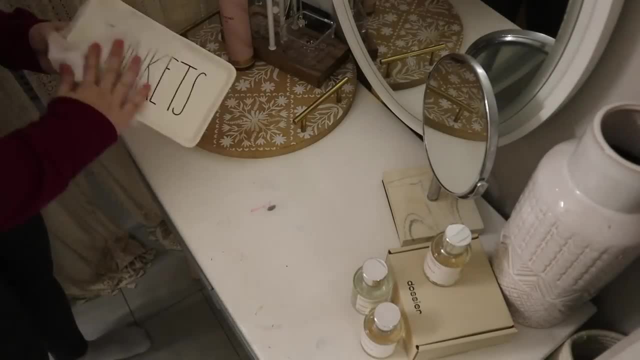 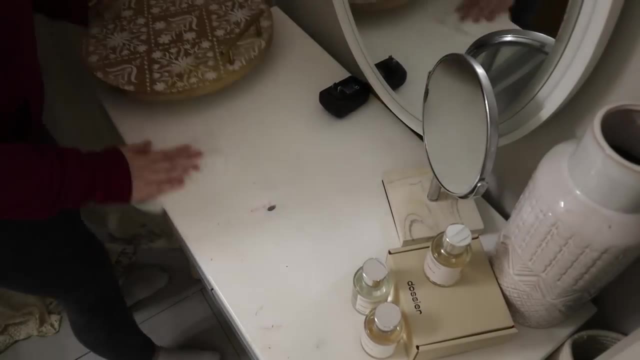 go through my closet. So stay tuned for that video because we will be taking care of my closet and getting that all organized very soon. Make sure to click on the subscribe button for daily��� crop pour videos. Find me on instagram: keepwa2000, 8 year old. 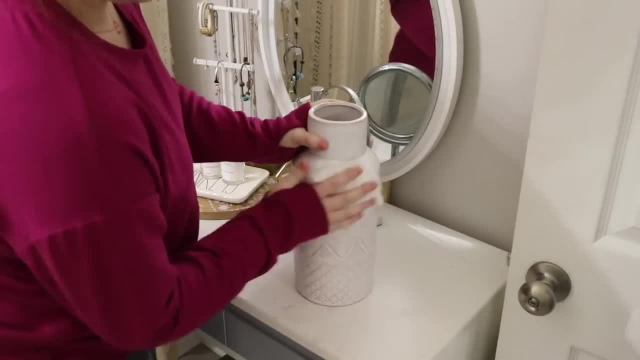 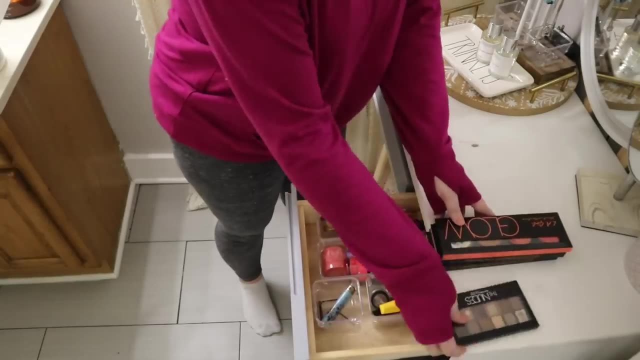 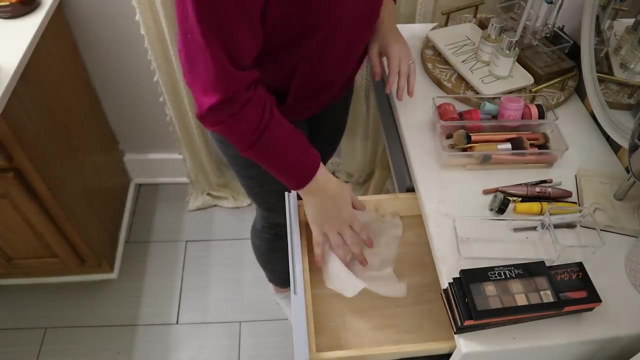 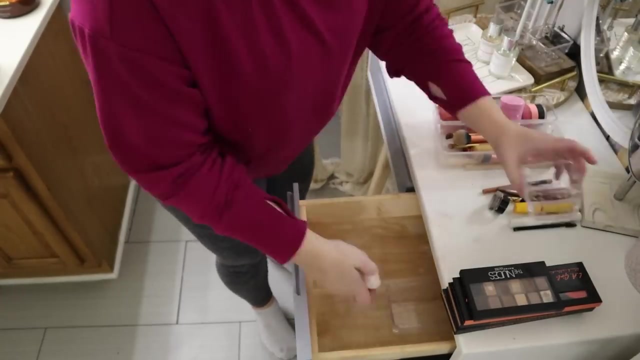 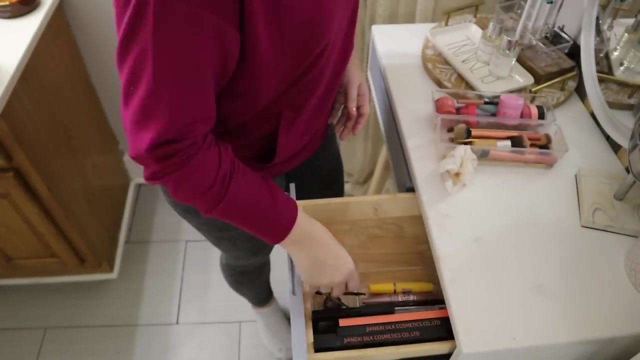 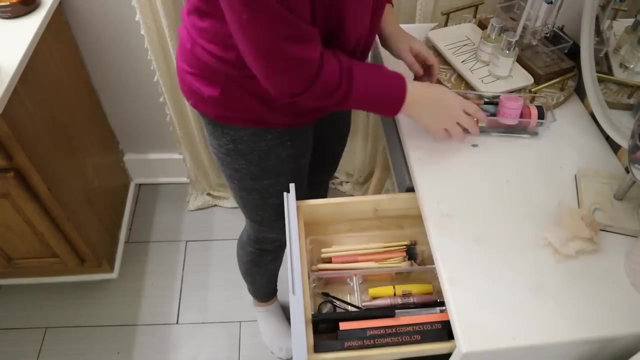 Here it comes. Oh, it is. the commissioner хочет найти kilometN IPhone, iphone, iphone, iphone, iphone. Ok, iphone, iphone, iphone, iphone, iphone, iphone, iphone, ipphone, iPhone, iphone, iphone, iphone, iphone, iphone, ipphone. I didn't have a lot to declutter out of my makeup vanity because I do keep that pretty minimal and 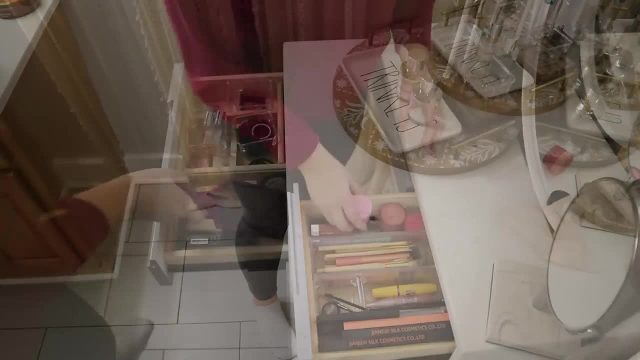 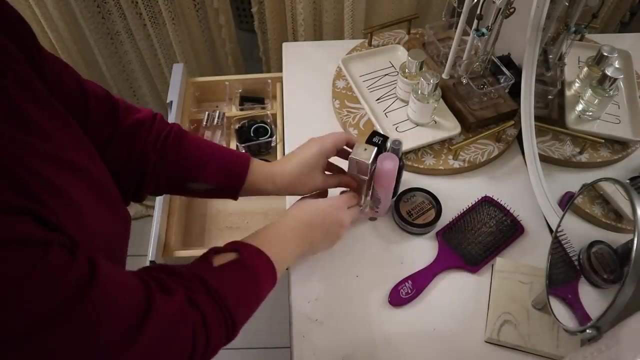 I usually am really good about throwing things away when I don't want it or it's running low, so I'm just going to take everything out. we're going to wipe that down. there was actually some makeup spilled like powder and just dust and all kind of stuff in here, so we're going to take all. 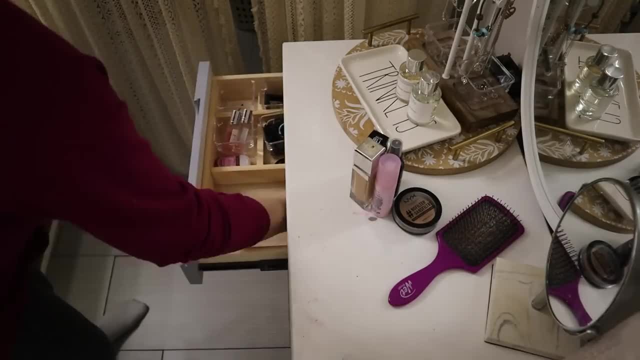 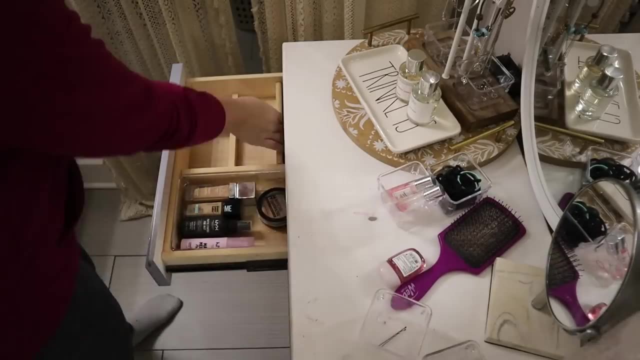 these acrylic organizers out and wipe those down. the acrylic organizers were actually dirty like needed to be wiped down, but the wood inside was pretty clean. but I just wanted to go ahead and just wipe it all down and start fresh with a clean slate and organize my makeup a little bit better. 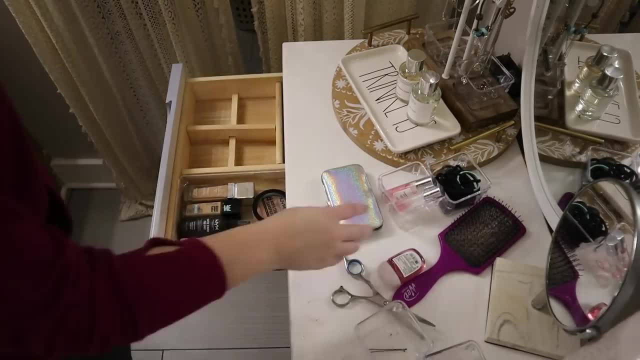 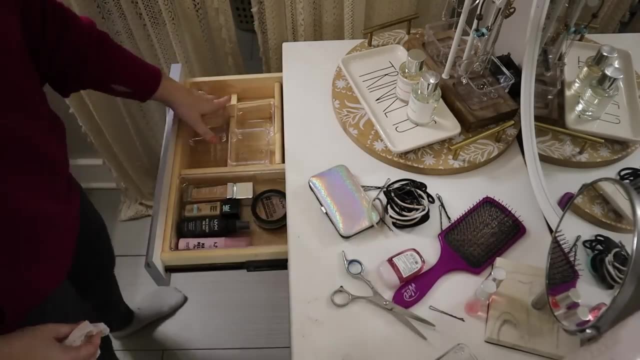 so do y'all collect a lot of makeup or do you only have what you wear on a daily basis? I will try out a new product here and there, but if I don't like it then I'll go back to what I was already using. or if I like it more than what. 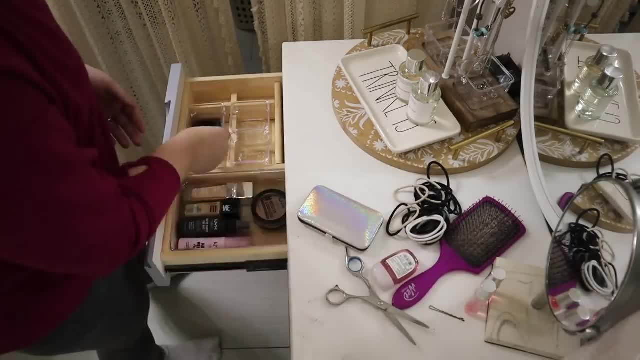 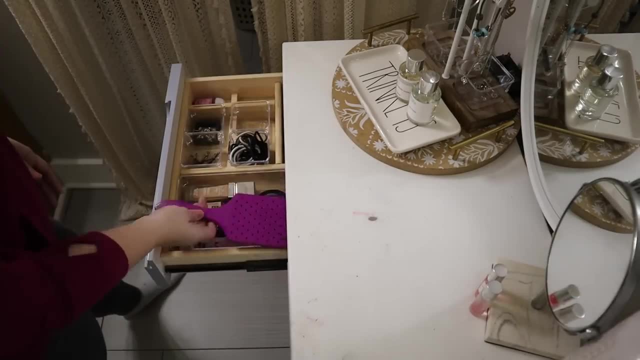 I was using, then I'll just start using that and start buying that. but I don't usually buy a whole bunch of makeup. I only have what I use. I'll have a little bit of extra, like date night style makeup, like darker lipsticks, but basically what you see is what you get right here. this is pretty much it. 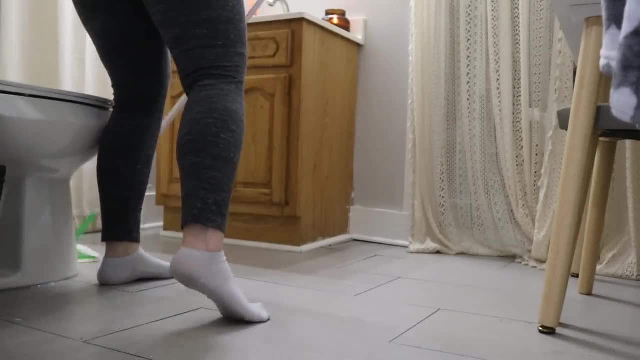 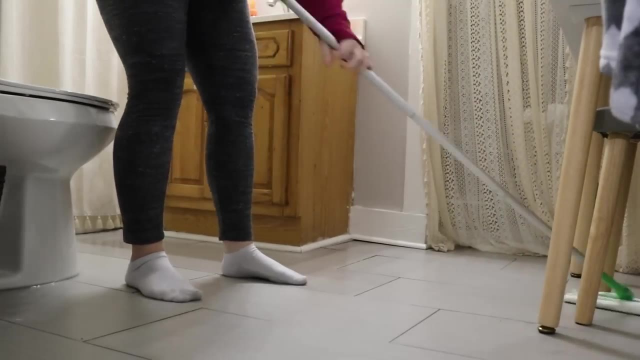 and also pretty much all of my makeup is drugstore. I usually get it all from either Target or Walmart and here in just a little bit, I'm going to be hanging that shelf that was in the kids bathroom over their toilet, in my bathroom over my vanity, and this was just like the missing. 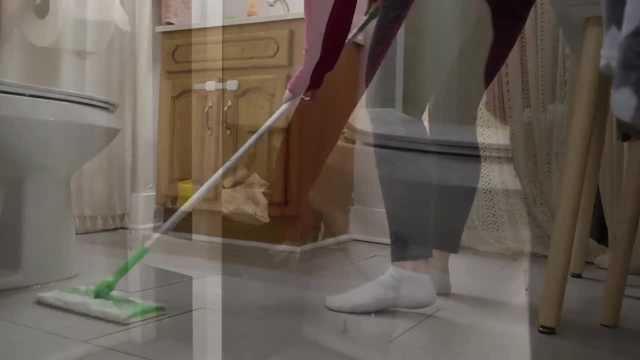 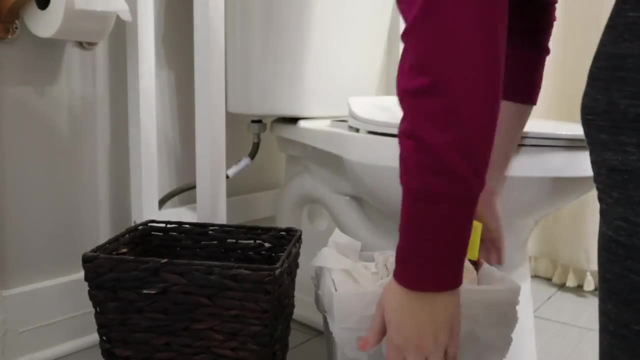 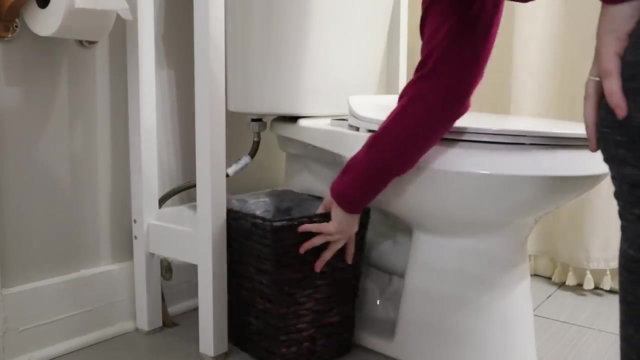 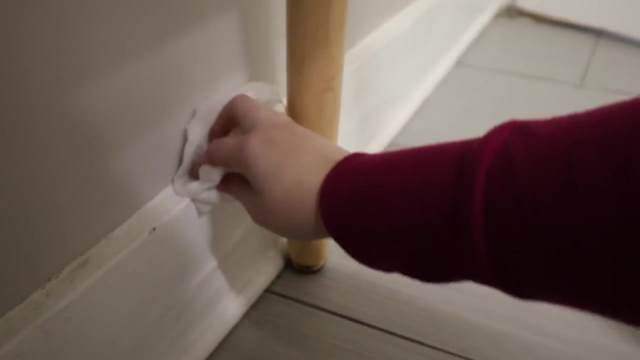 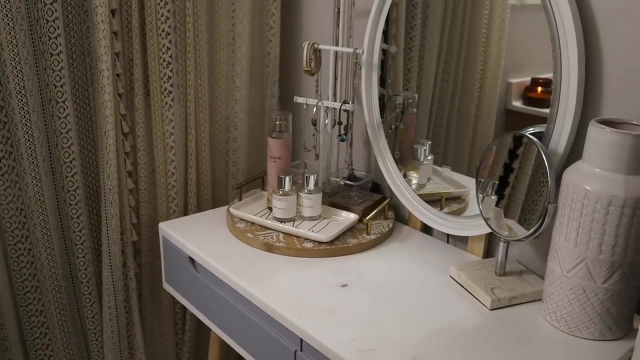 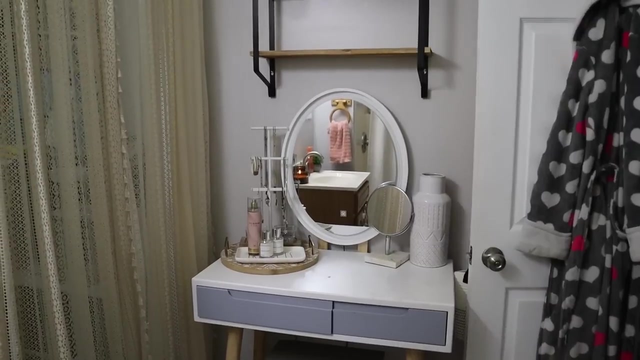 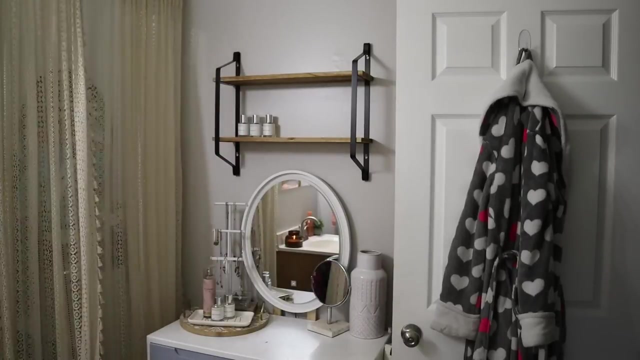 piece to my puzzle. it looks so good in here and it was so helpful- I was able to put all of my perfumes on it, so we are going to take care of that here in just a minute. I know y'all have heard me talk about dossier a lot, but I am putting all of my dossier collection. 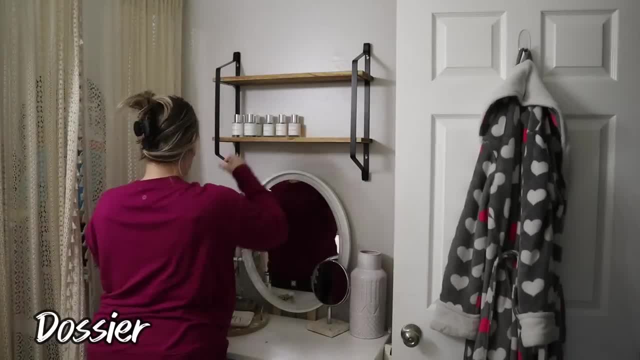 perfumes here on my shelf. I love these perfumes because they just look very acidic and, like I said earlier, I love these perfumes because they just look very aesthetic and, like I said earlier, I love these perfumes because they just look very acidic and, like I said earlier, not everything has to look. 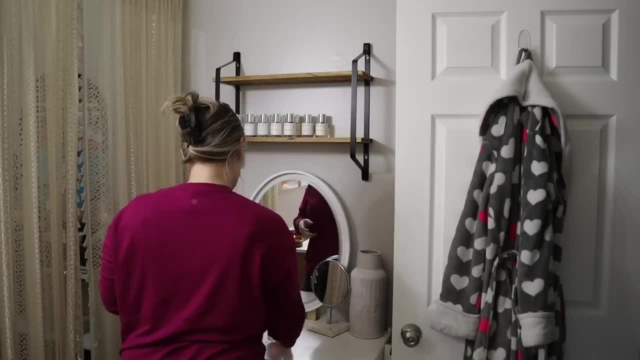 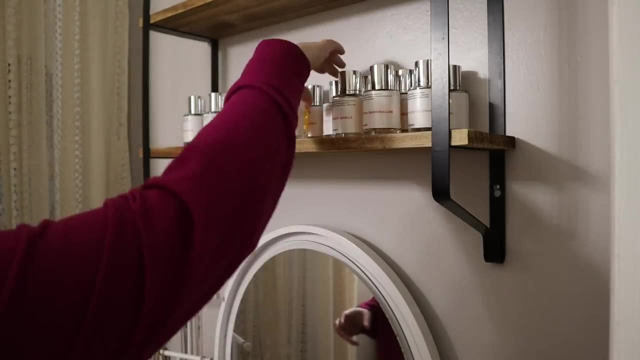 aesthetic, but you can make it look nice. but I do love the way that all these perfumes look when they're all side-by-side, so I'm just kind of putting my same scents in front of each other. so I basically have two of each scent and then I only have one of the coconut scent for summer. so 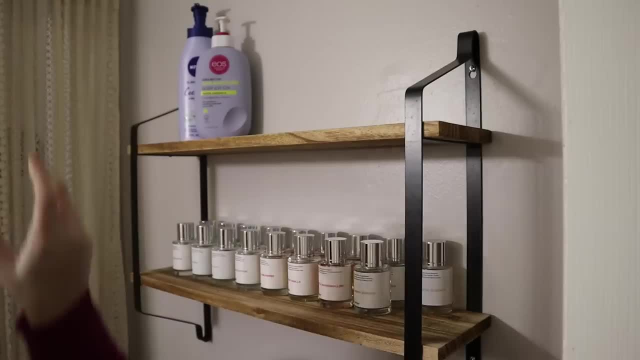 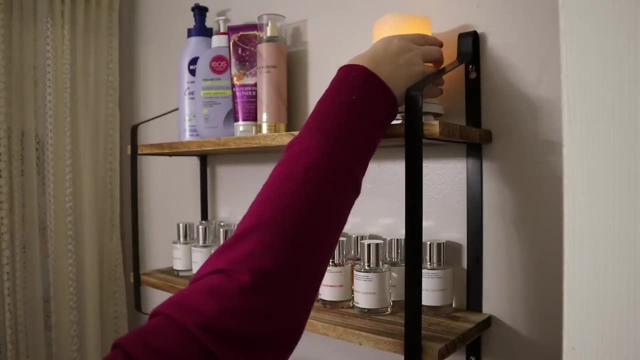 I will have to get one more of those. but if y'all are interested in the dossier perfumes, I love this line. I love this brand. dossier is a luxury inspired a fragrance brand. they sell higher-end perfumes for a much cheaper price. and I love this line. I love this brand. dossier is a luxury inspired a fragrance brand. they sell higher-end perfumes for a much cheaper. 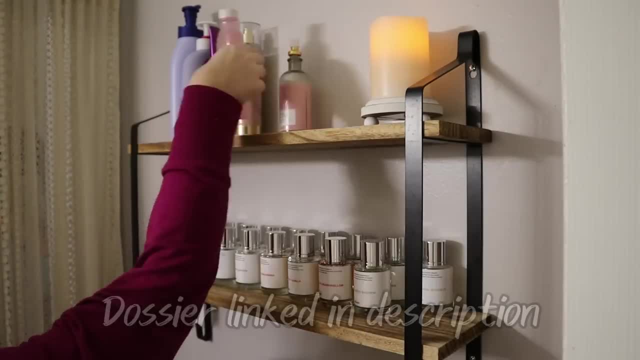 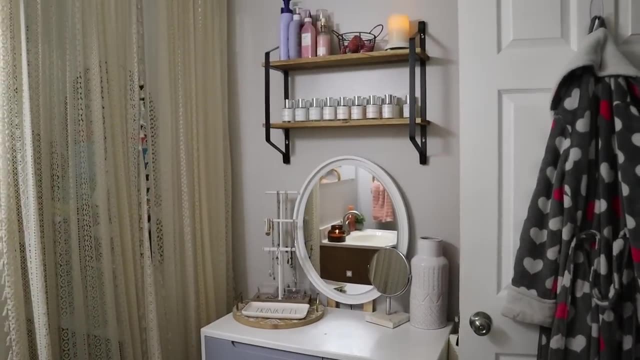 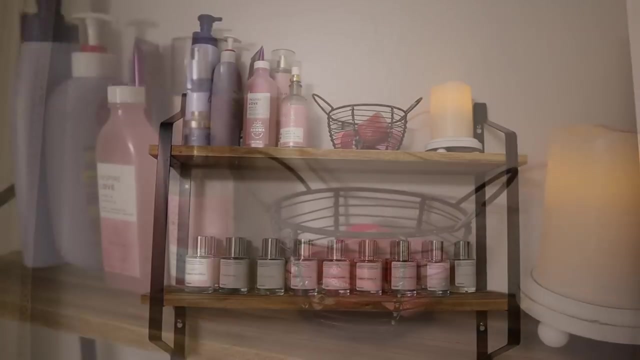 price tag and if you don't like the perfume that you chose online, then you can return it for a full refund, no questions asked. and you can also check your local Walmart, because select Walmarts also sell dossier perfumes in store and they have scents for women, men and unisex, and I do have several. 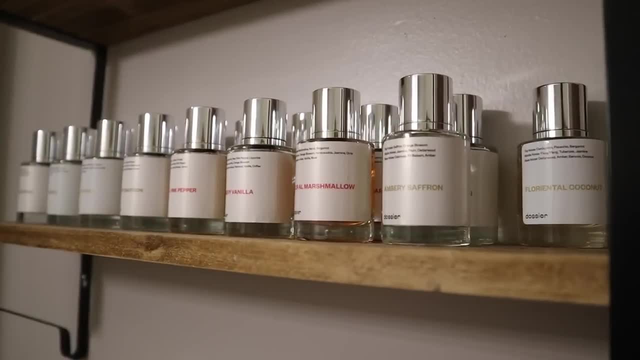 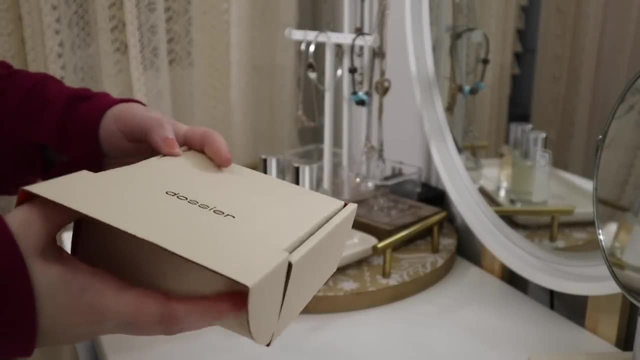 favorites that I have shared with you guys. with Valentine's Day coming up, I can highly, highly, highly recommend the citrus marine for your man. it is the one that my husband wears a lot. I love that scent for a man. it smells amazing, you guys. so definitely check out citrus. 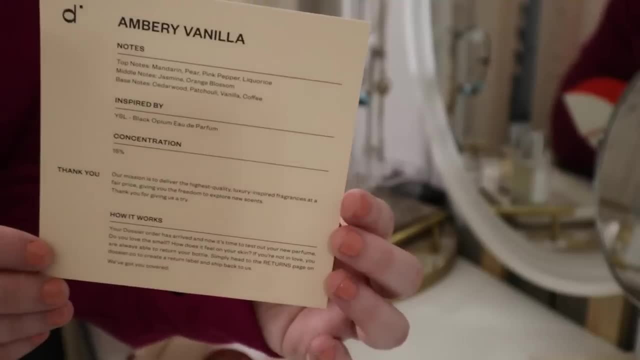 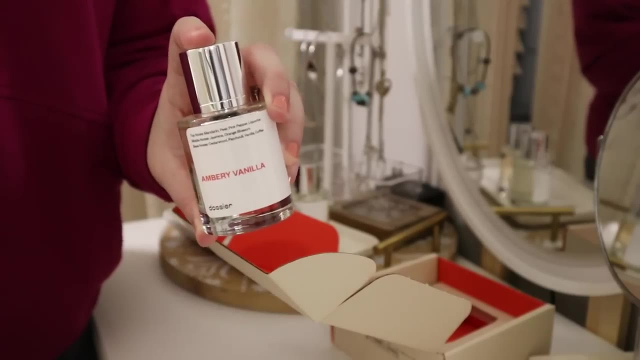 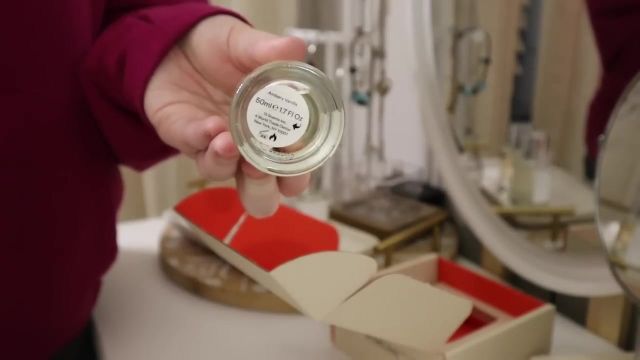 marine for your man. and then every perfume is gonna come with a note card. this one is the amber e vanilla. this has been one of my favorites lately. I have shared it multiple times. it smells like an iced vanilla latte in a bottle. you get a 50 milliliter bottle with a magnetic snap-on lid so you don't have 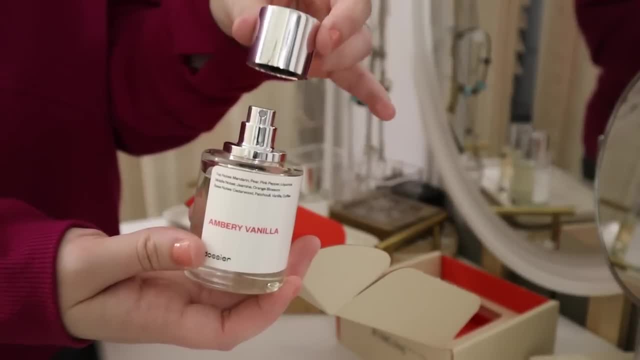 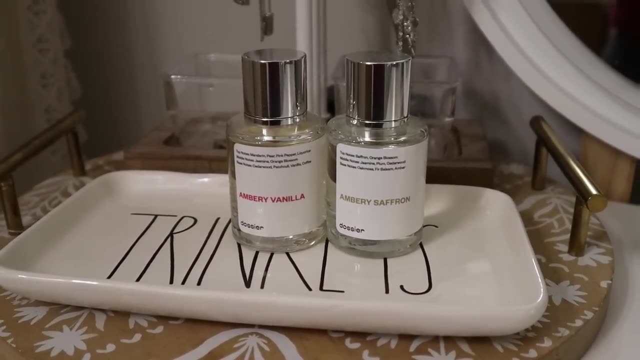 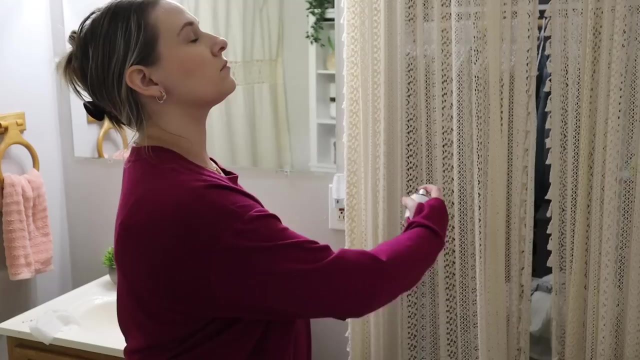 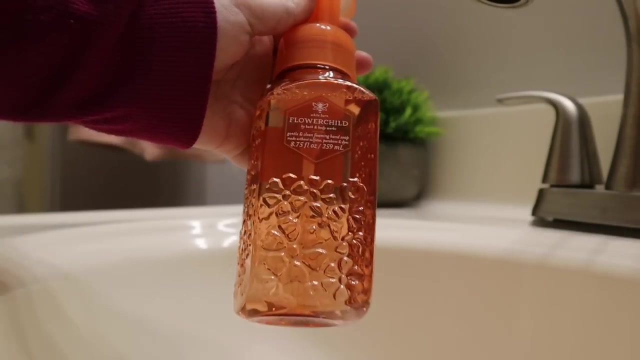 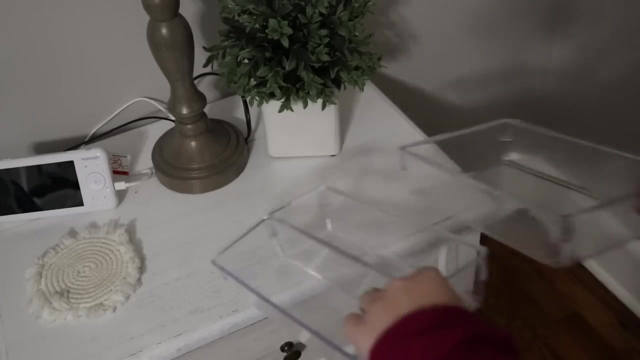 to worry about it leaking in your car or your diaper bag or your purse. and you guys, something that I love about dossier is that the all the perfumes that are sent back to them, they donate them all to charity, so no bottle of perfume ever goes to waste. another favorite is the amber e. 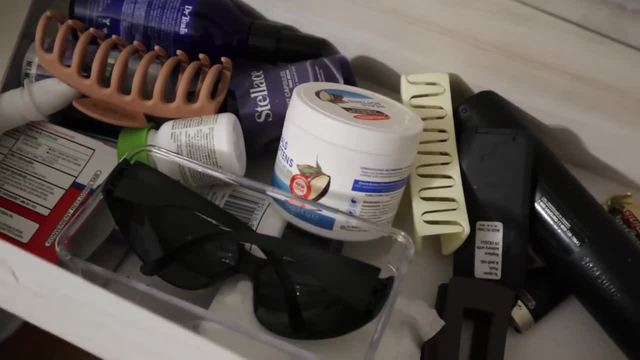 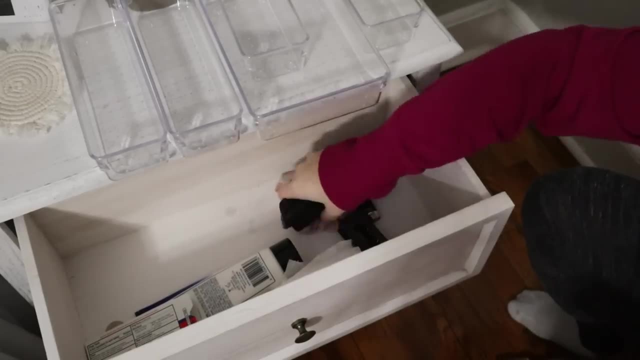 my favorite spring scent this year. So let's go ahead and head into my bedroom. I'm going to tackle my nightstand. It has gotten out of control. I was trying to fit all of these acrylic drawer organizers in my nightstand, but it just unfortunately did not fit. The top drawer is 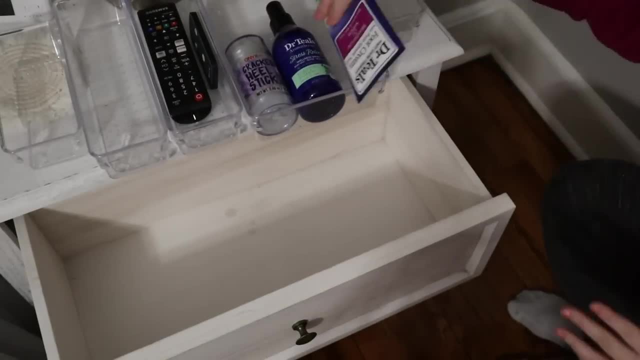 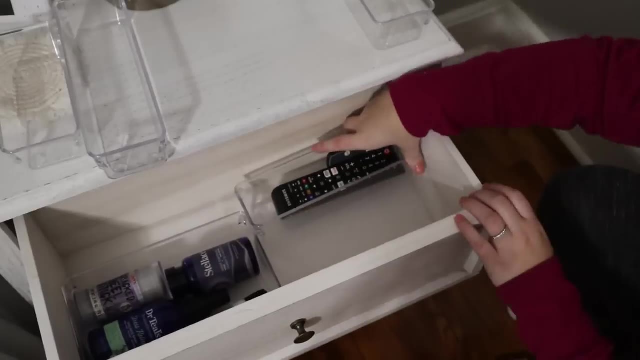 smaller than the bottom drawer. The bottom drawer: I keep my important folder and I have a heating pad in there and that's pretty much all that I keep down there. But my nightstand was incredibly unorganized and it was bothering me, So we're going to go ahead and take care of that. I decluttered. 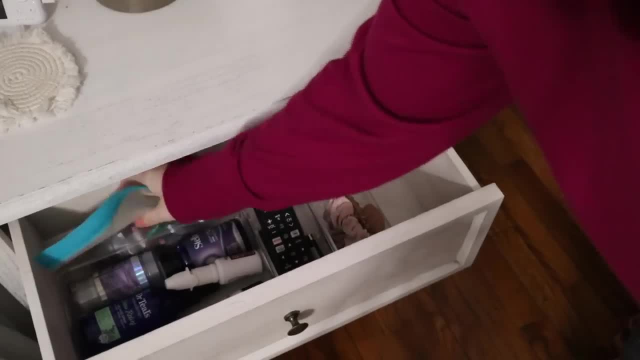 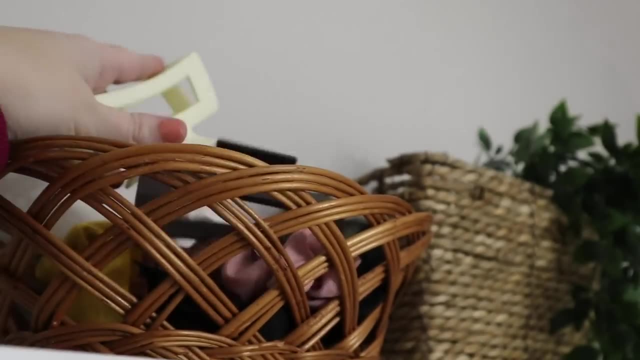 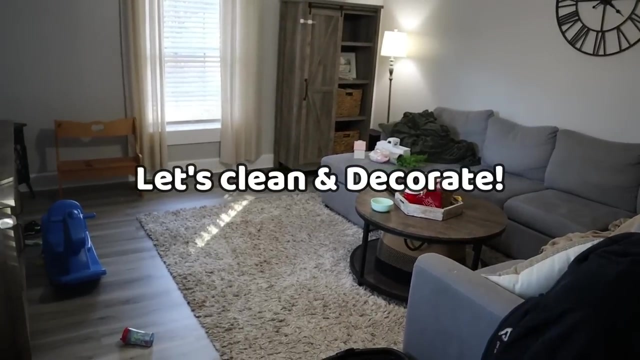 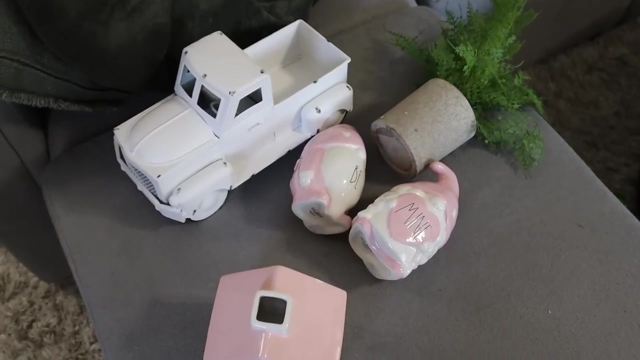 a lot of stuff out of here. I put things back where they go and made it so much more simple. And also I have a little treat bag in there because you know mama's got to have her stash. So over here on my bookshelf. 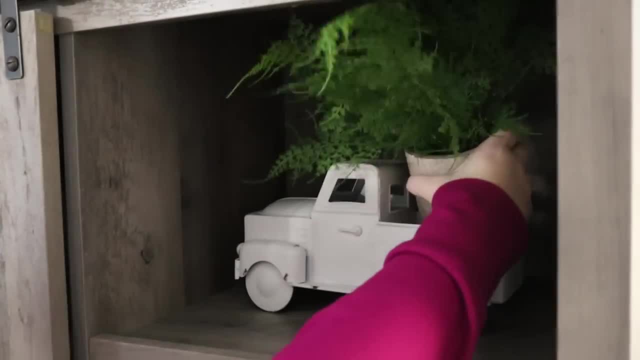 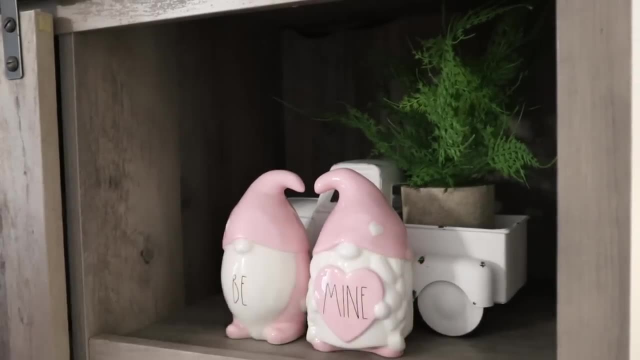 I wanted to add add a few little pops of Valentine's Day In my Valentine's clean and decorate video. I was trying to keep it super simple and not go all out with Valentine's Day and there's a few pieces that I didn't use that I decided I wanted to use. So I'm just going to add my Be Mine gnomes to the top. 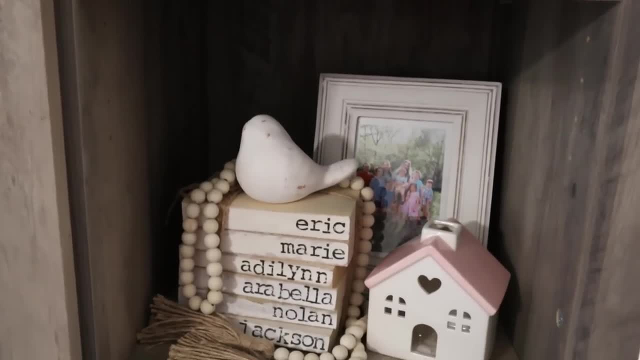 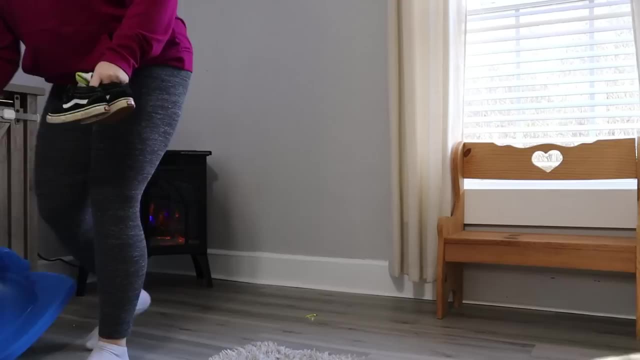 shelf with my truck and in the second shelf down, we're just going to add this little house with the pink roof. I love using pops of pink for Valentine's Day over red, just because I use so much red for Christmas. My house in the living room was a complete disaster. My kids had pulled. 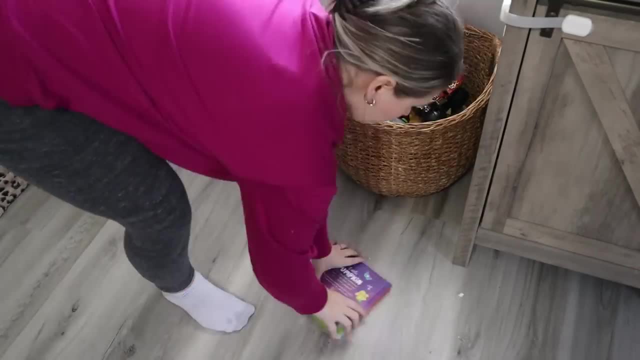 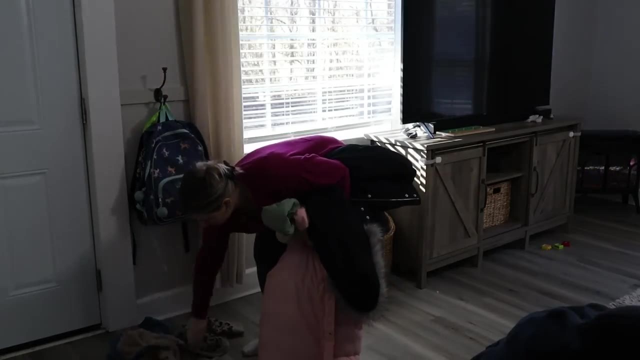 all their toys out. They were strode all over the place. There were coats, book bags, jackets, everything everywhere. It was giving me so much anxiety, so we're going to go ahead and take care of it. Also, if you look over next to my tv, I do have a new little space heater fireplace. It looks 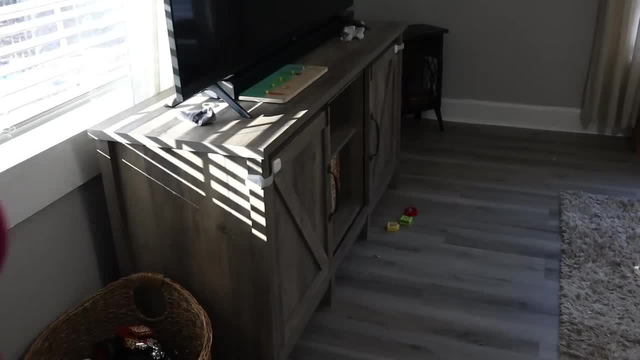 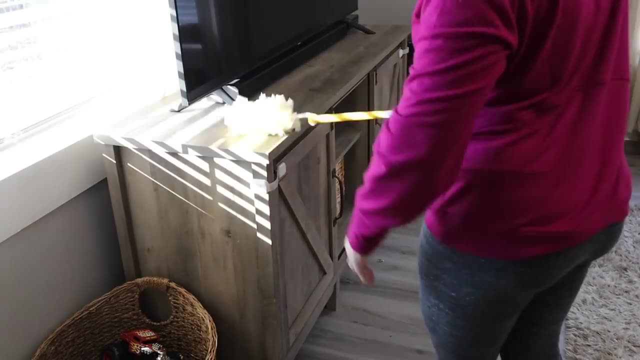 like a real fireplace. I found it on Amazon and it warms up the house so good. It works really well. It goes to low, Or you can put it on high or you can just use the fireplace and turn the heat off if your house is. 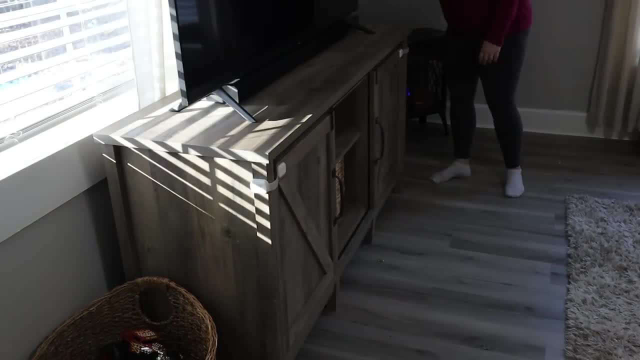 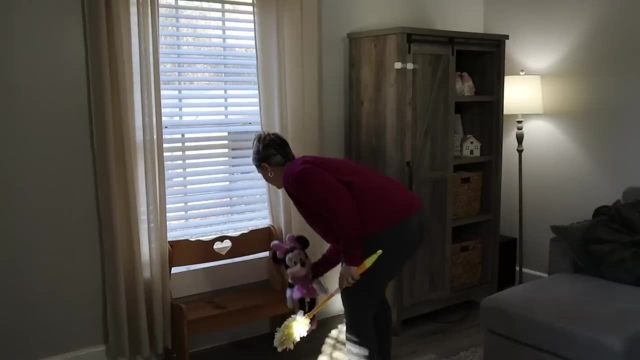 warm enough. So if y'all are interested in that little space heater, I will have that linked below, but I love to go stand in front of it when I'm cold. It's so nice, warm and toasty and we've all been really enjoying it. And I found that little bench at Goodwill. They had it priced for $25. 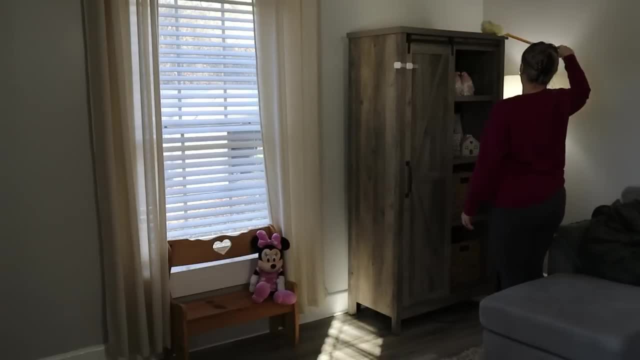 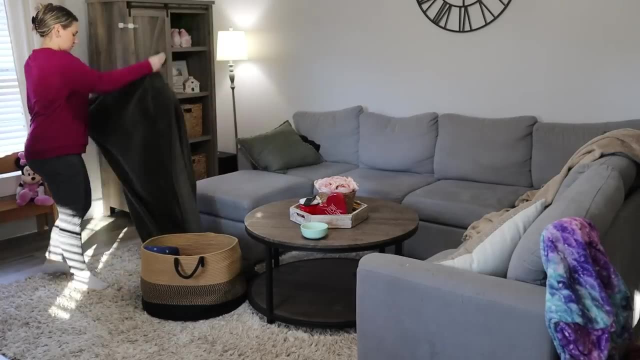 and I had went back and they still had it and it was 50% off. So I got it for about 12 bucks, you guys, and that was such a good deal. I love that little bench. The kids have been sitting on it and playing. 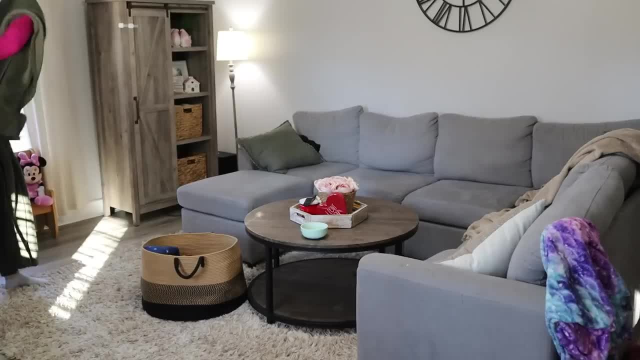 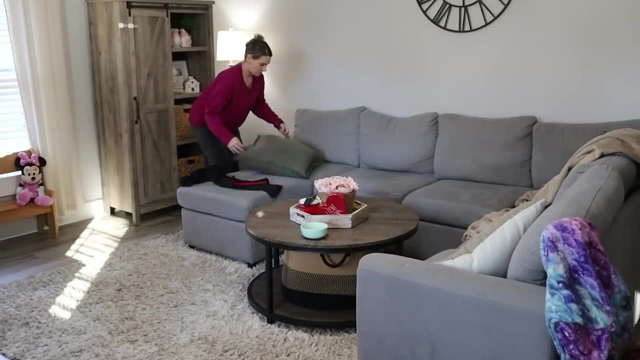 And they just love to go sit on it. But I just think it is so adorable and I will let y'all know that this video is going up a little bit backwards, So my next video will actually have my Goodwill haul, where I went to Goodwill and I got a few things, But I needed to post this video first. 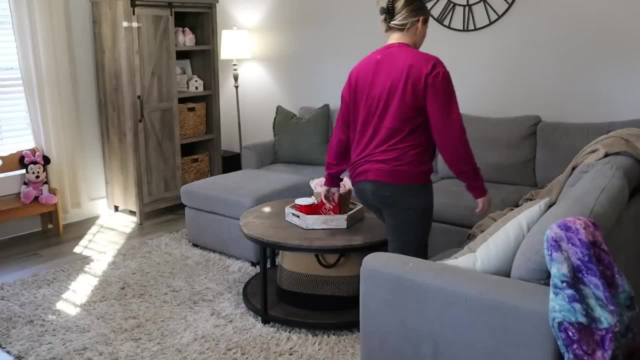 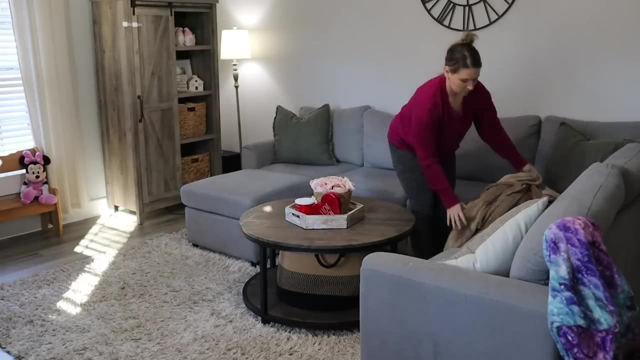 because I needed my dossier feature to go up. The dossier perfumes are sponsored, you guys, but I do. I do really love them, I genuinely enjoy their perfumes and I've said it before, but I will never share anything on my channel that I don't genuinely love or use. So if you guys are interested in that, 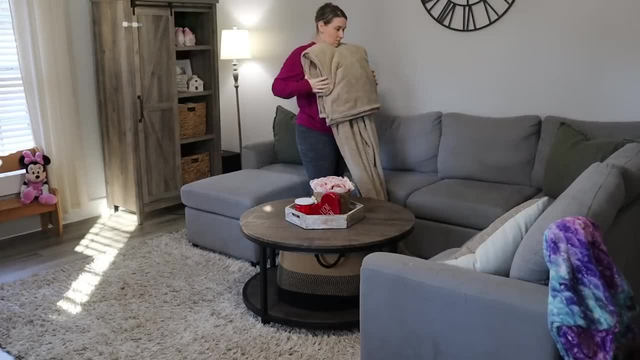 please let me know in the comments down below. And there have been things that I've received from companies that I didn't really like and I let them know and I did not feature them. So definitely keep in mind that when I do share something on my channel, it is something that I really like. 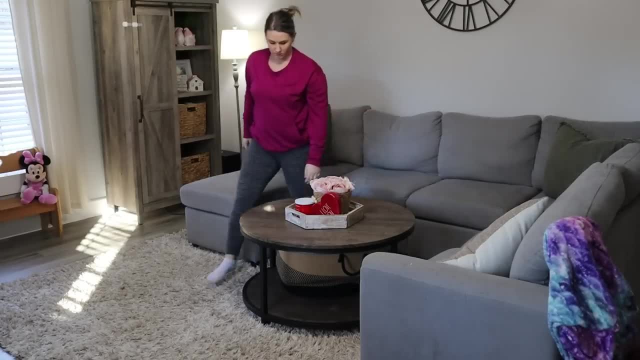 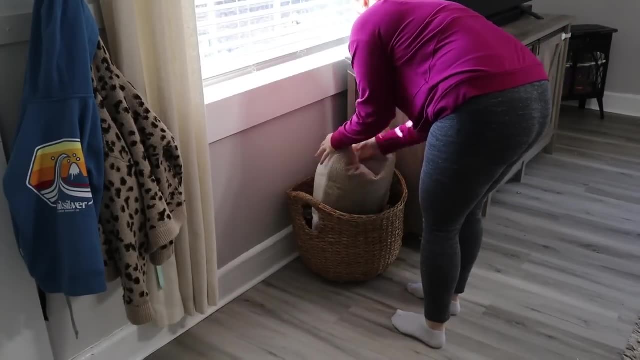 So I actually had some packages behind the couch. They are mattresses from my boys room, because we are about to make over the boys room, you guys. That's going to be such a fun, exciting video. So baby Jackson is going to be practicing sleeping in a toddler bed. We're just going to take the 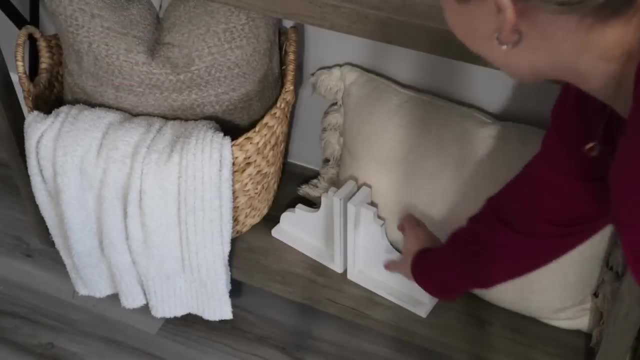 first one, and we're going to take the second one, and we're going to take the third one and we're off of his crib and let him practice sleeping in his bed that way. I know it's going to be a few restful nights because you know you got to train them. But once he's good and trained and used to, 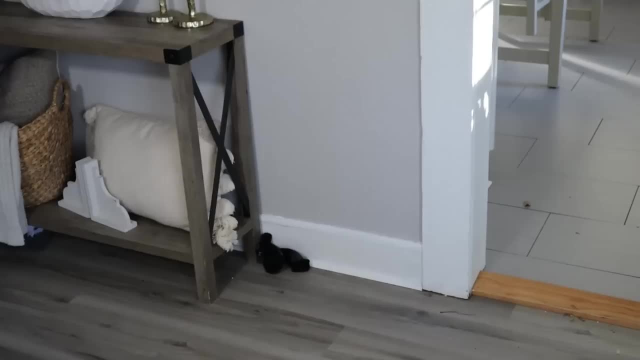 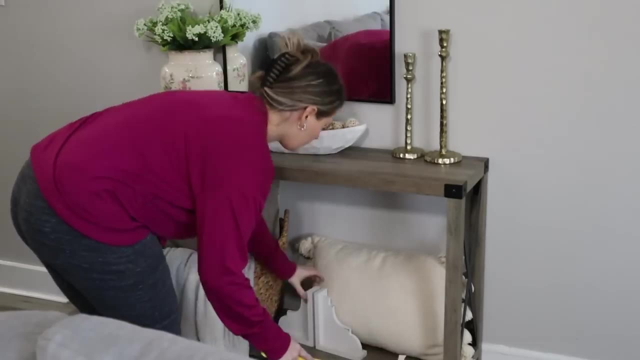 that we are going to take these mattresses and new beds and we are going to do the cutest theme ever. So definitely stay tuned for that video. y'all And y'all have to let me know what age did you change your kids to a toddler bed and what methods did you use to keep them in their bed. 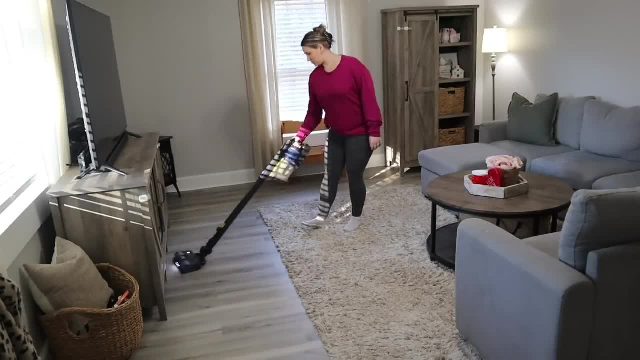 This is my fourth kid, so I do have experience and I do have a lot of experience. I do have a lot of experience and I do have a lot of experience. I have my own little techniques, but I would love to know what worked for y'all and maybe I can. 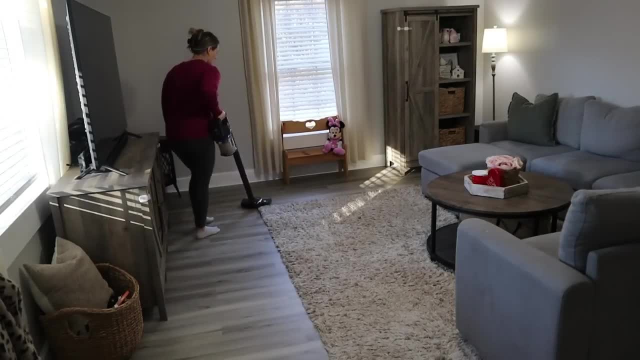 incorporate those into the way that I keep my kids in the bed. Basically, I just keep walking them back to the bed, telling them: no, no, it's time to go to bed, And I also like to keep a baby gate up just for safety, so they can't run through the house in the middle of the night all alone. 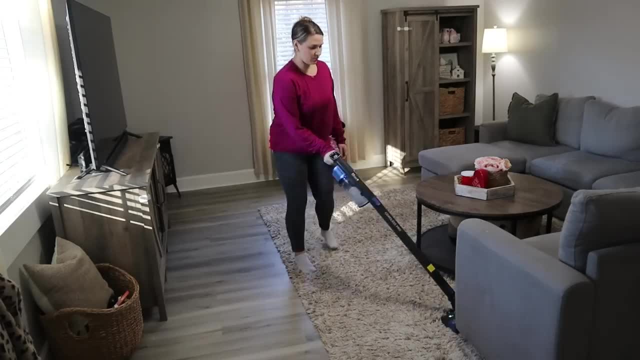 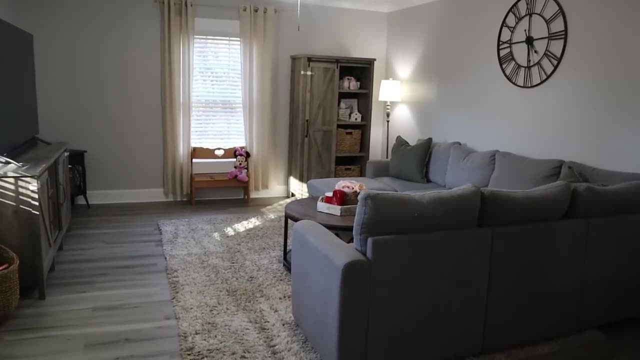 So, anyways, I'm going to finish cleaning up and decorating in my living room. I also have these gorgeous beads that I'm about to add to my coffee table. I had some beads on there, but they are so small, And I found some big fat beads at Goodwill for so cheap. I think they were like: 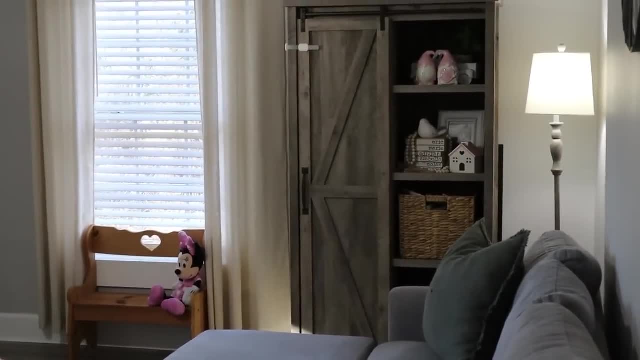 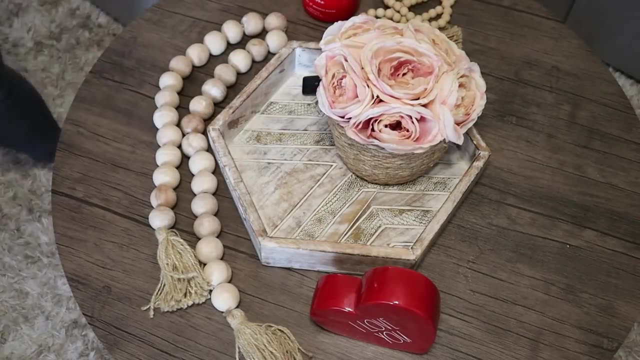 four dollars or something like that. They were so cheap, And the ones at Hobby Lobby are like thirty dollars or just like overpriced. So I cannot contain my excitement that I found these beads. I'm so excited I found these. I love the weathered look of them. But I'm just going to wrap these. 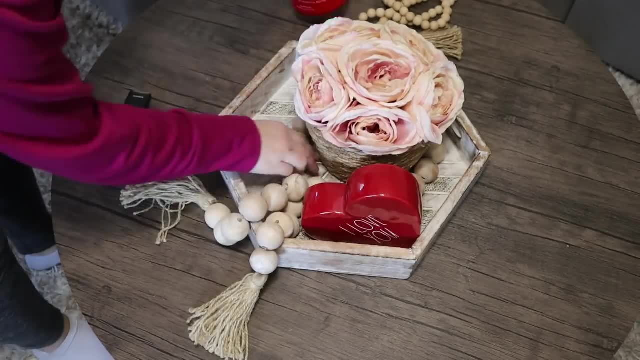 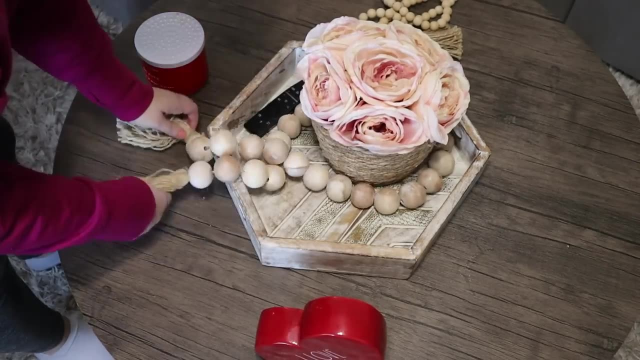 around my roses and put my decor back on the tray And I just love this big, fat bead so much It makes me feel good And I'm going to add a few beads on top of this one to put on my table. But I love these. I think they're so gorgeous. Sometimes when I go to Goodwill I don't see. 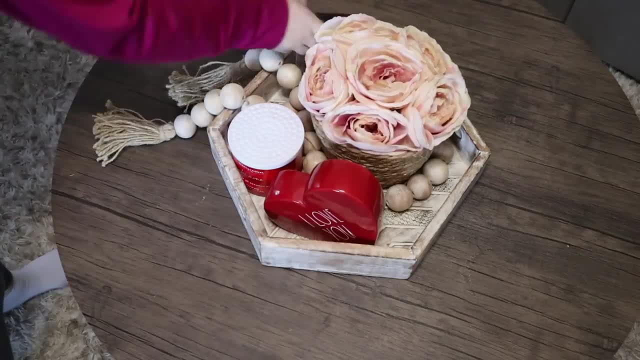 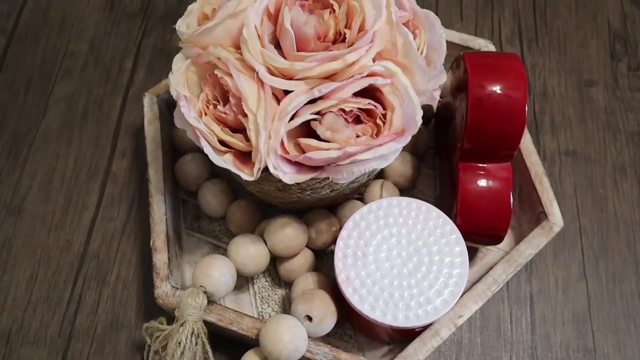 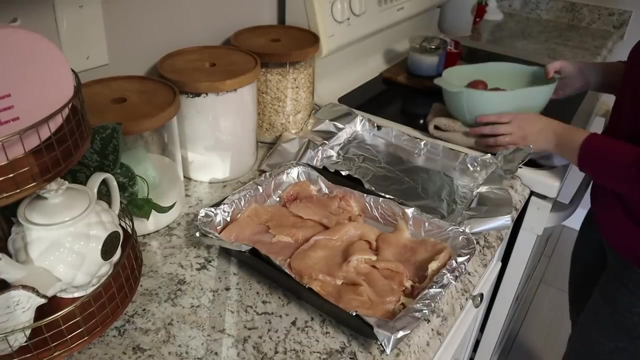 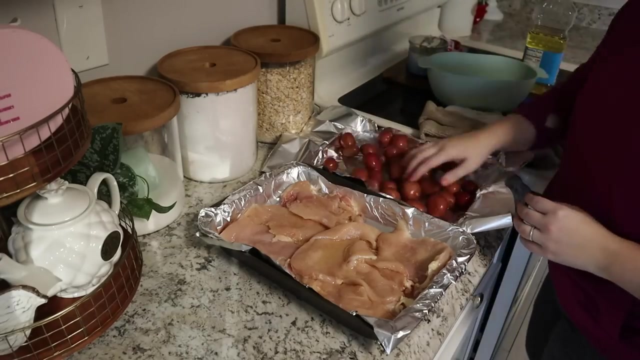 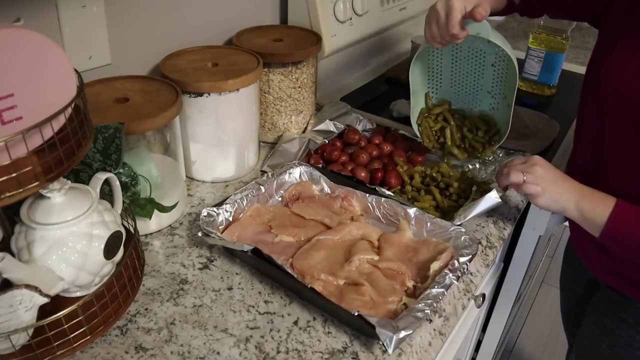 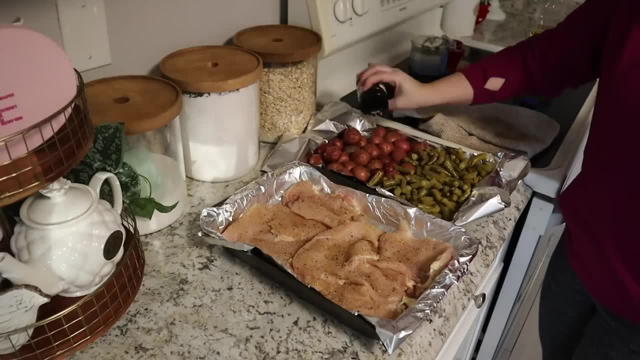 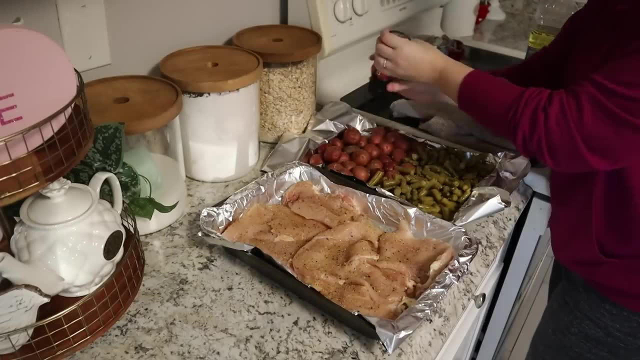 to add the blend, which is salt, pepper and garlic powder. we're going to add this to all of the potatoes, the green beans and the chicken, and i'll have to use a lot of chicken, a lot of green beans and a lot of potatoes because we're a family of six, but if you're a smaller family, you can. 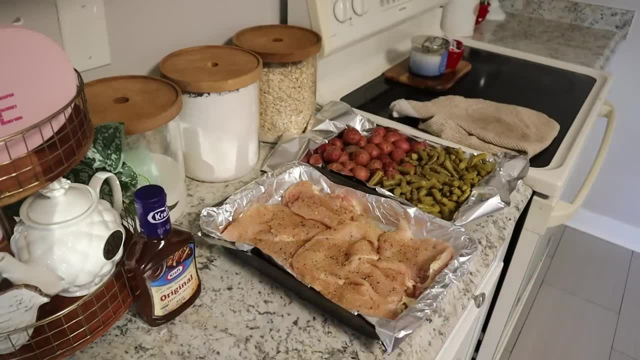 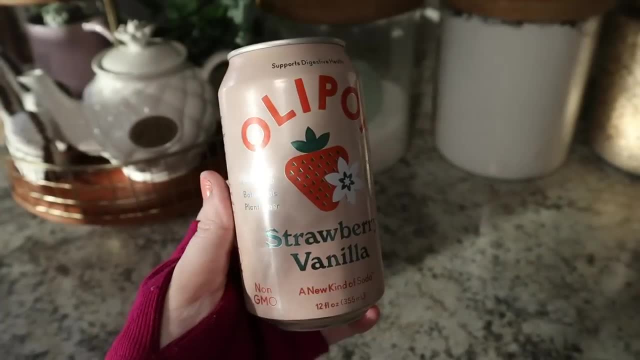 fit all of this into one pan. i'm also going to be using some italian seasoning. i'm not going to cover my chicken, but i am going to cover my potatoes and my green beans. we're going to cook this in the oven on 375 for an hour, and it is so good and easy. and while that's cooking, i'm going 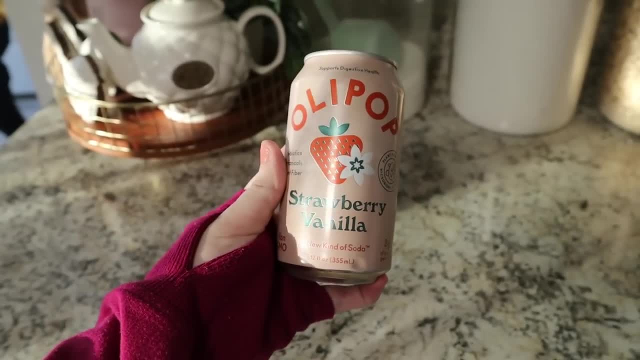 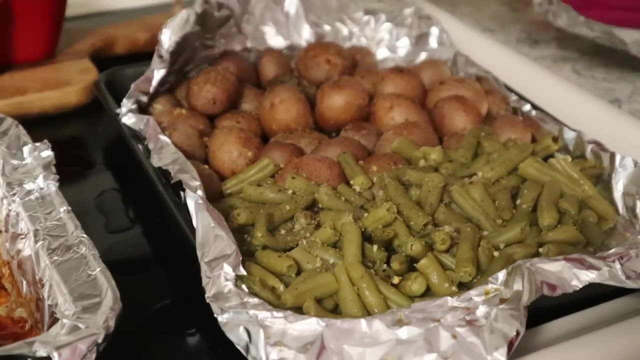 to grab me a strawberry vanilla soda. this is a healthier soda that i've been drinking. i know a lot of people know about these, but these are so good. i have got them a while ago and i just completely forgot about them. and then i remembered about them again. 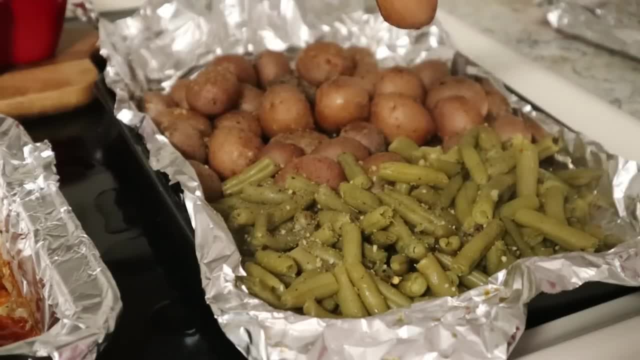 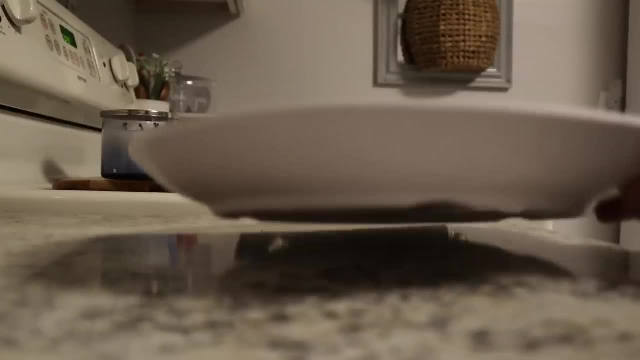 recently, so i picked those up from the store. but this is the way our dinner turned out. it was so, so yummy and a must try. such an easy dinner for tired mamas. it doesn't take long to prep it. just make sure your meat's already thawed out and you can throw everything in the pan and stick it in. 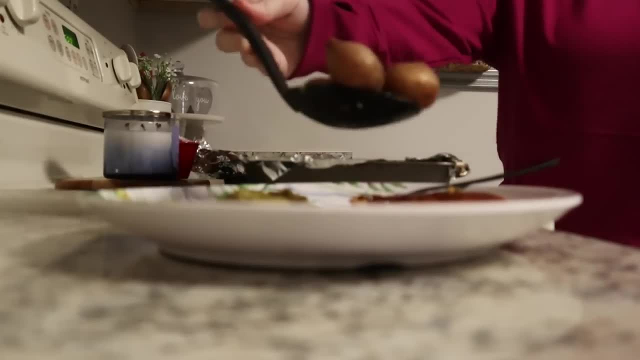 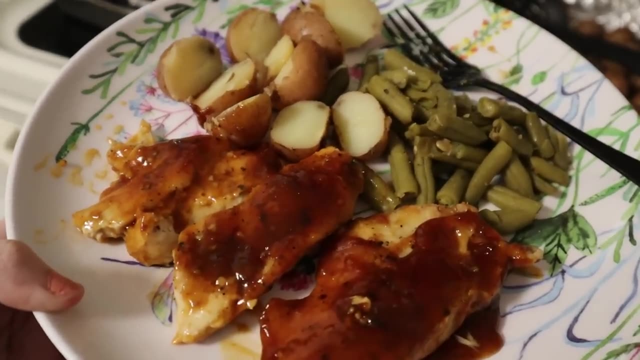 the oven and on long days like this, when you're doing a lot, you will thank yourself that you have an easy dinner. and last but not least, i'm just going to organize through our medicines and put together a little first aid kit to keep in our cabinet. so i'm going to go ahead and take care. 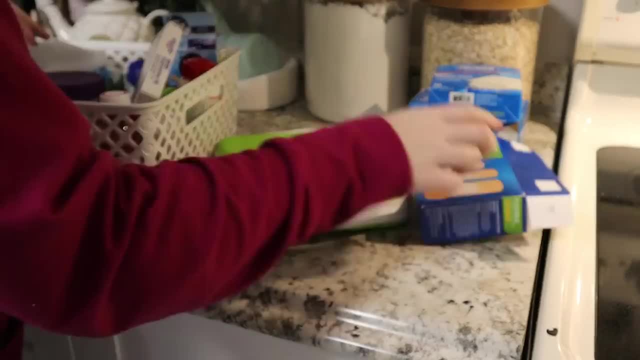 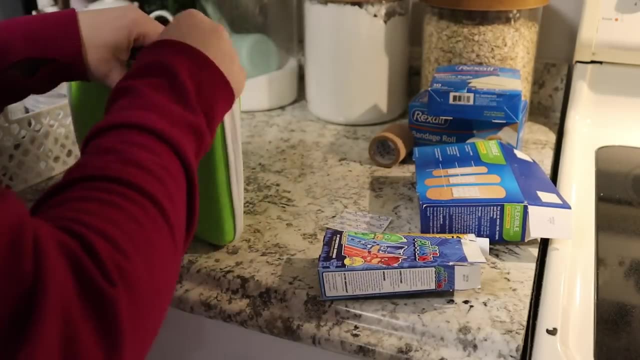 of that and i'll see you guys in my next video, and thank you so much for watching today's video. i hope it motivated you to get some stuff done in your house. subscribe if you're new- i would love to have you, and i will see y'all in my next one.